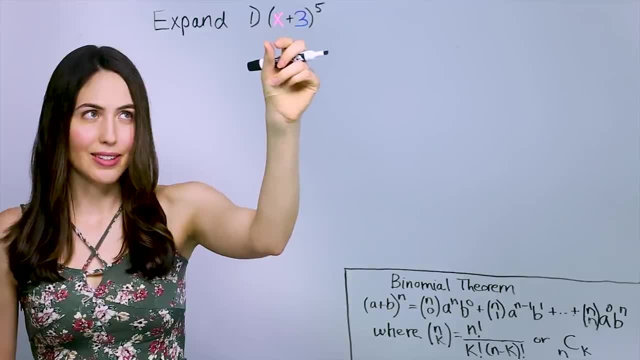 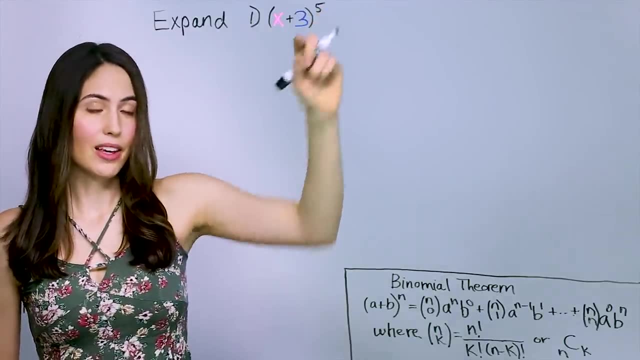 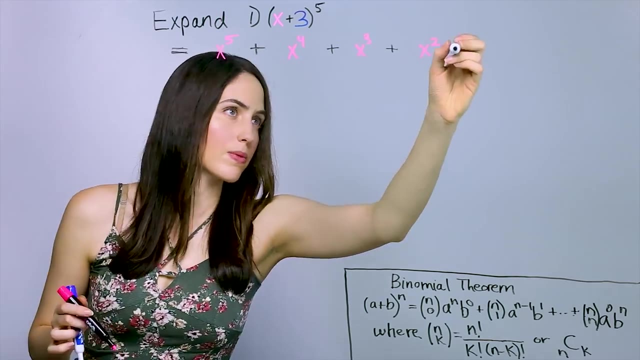 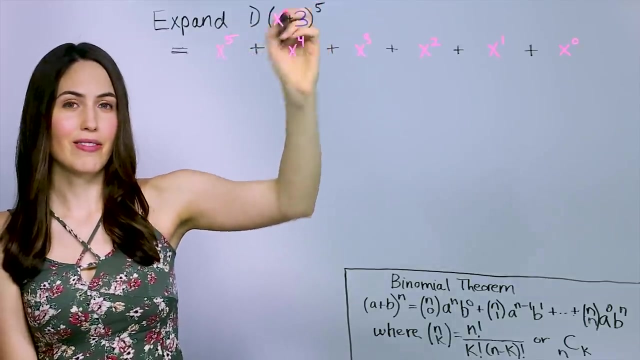 The pattern. we take the first part, x, and it will start with a power of 5,, our power number, and then go down by 1 in each term of the expansion. Okay, so the powers of x, the first factor, start high at our power of 5,. 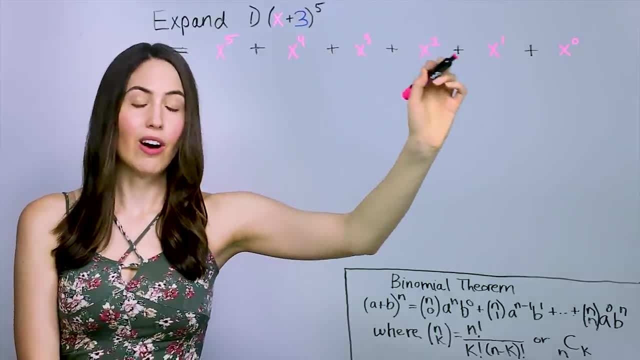 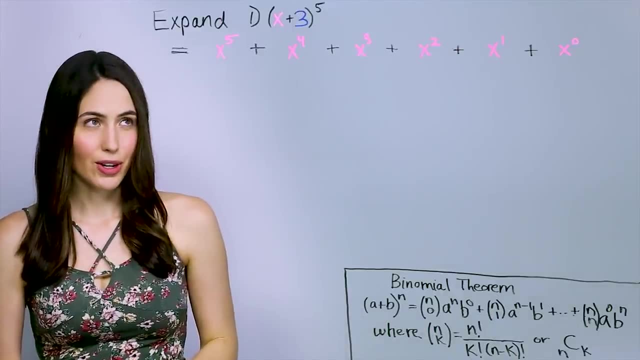 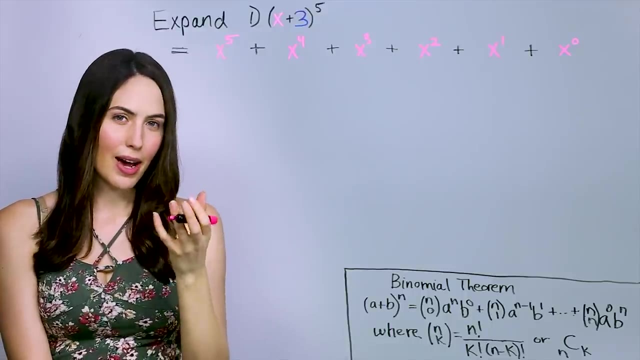 and then decrease by 1 in each term of the expansion, all the way down to 0.. Not 1,, but 0.. Now for the second term. our factor of 3 is going to start on the low end at power 0, and then go up by 1.. 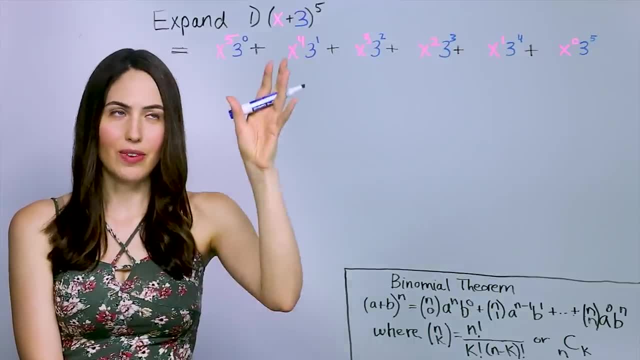 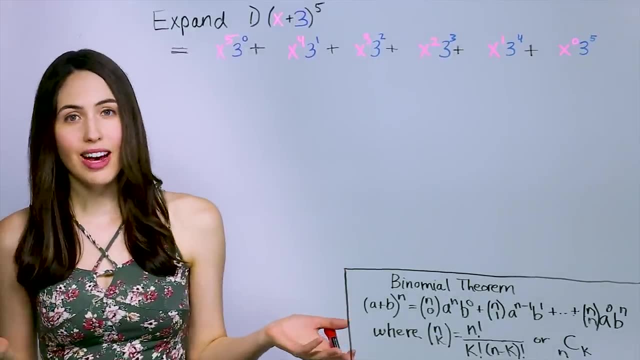 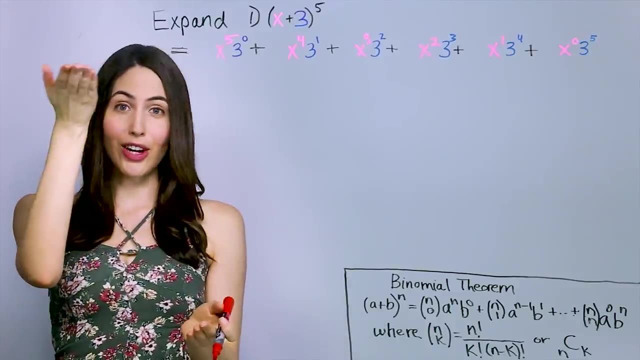 So you can see for that second factor 3, it starts low and then increases by 1 in each term. Alright, so that's a pretty good start. I mean, you're basically halfway done with your expansion. One thing: notice how these powers are shifting. So the power of x starts high and goes low. 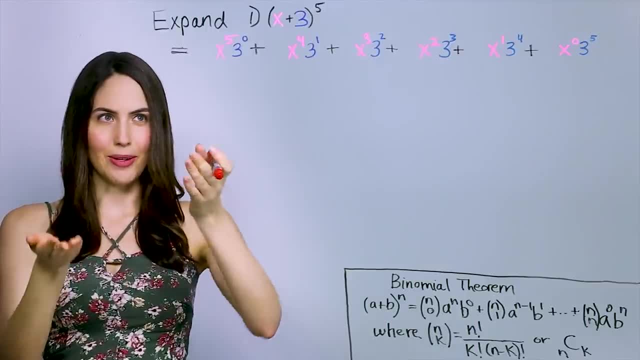 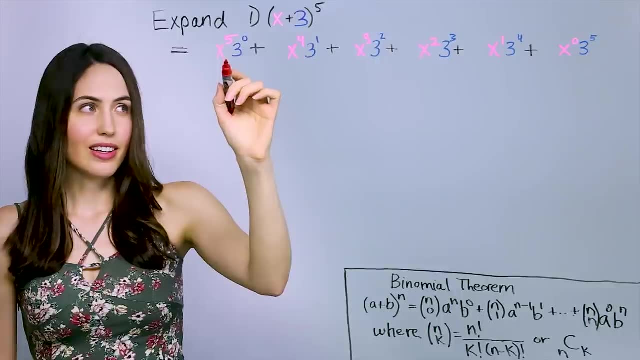 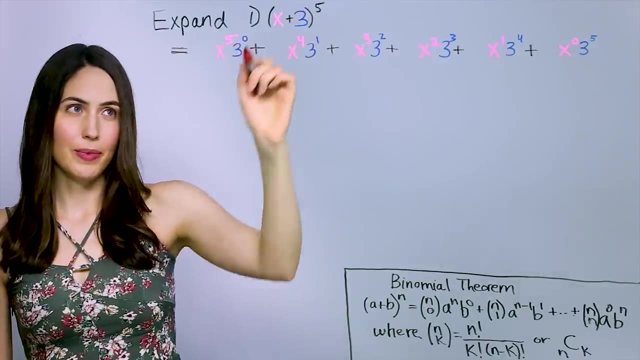 Power of 3 starts low and goes high, So they're going in opposite directions. They're shifting one by one. though, if you see what I mean For each term, notice how, if you add the powers, it's always going to add to your power number five here. 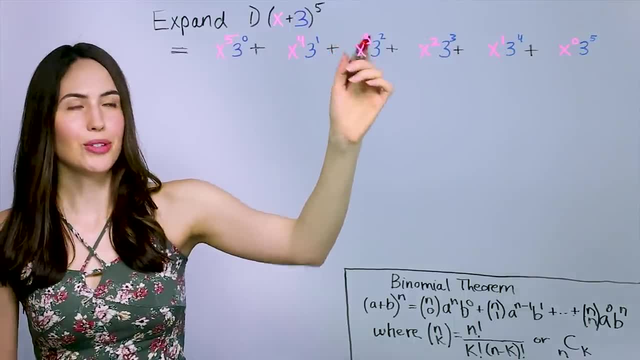 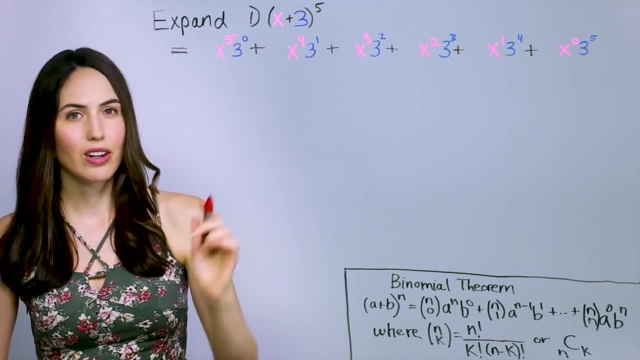 so five plus zero is five. four plus one is five, three plus two. it's always going to be true in these, And also one thing: you might think that for an expansion raised to power five, that you would have five terms. 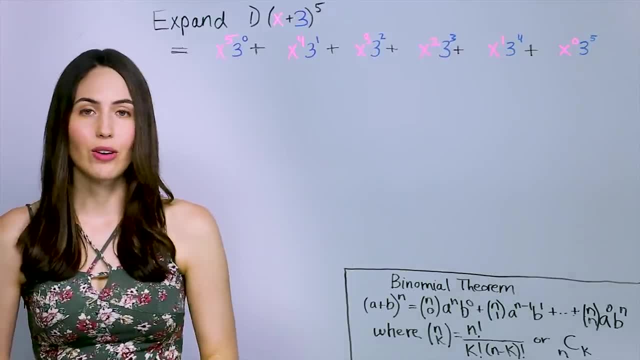 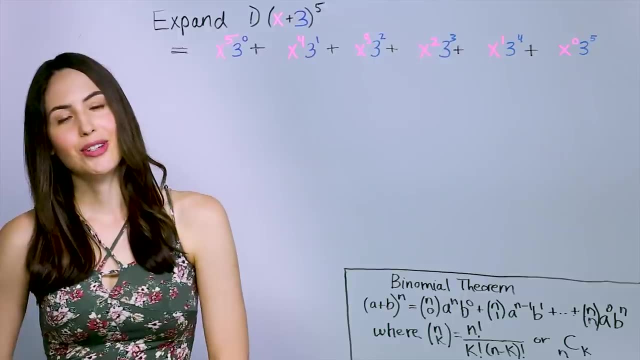 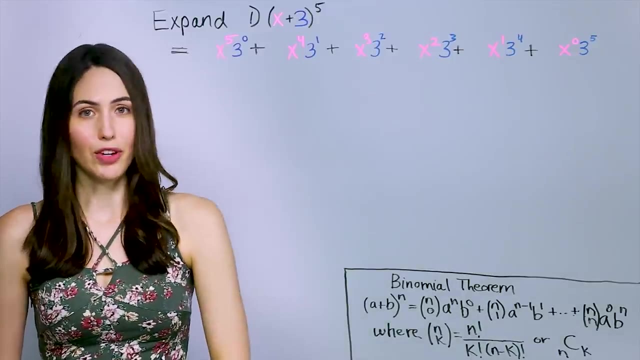 You actually have six terms. if you count them, It's just because we're doing the whole counting from zero thing is one more term than you would think. Okay, so we're not done. unfortunately, There's one more number that gets multiplied in front of each term, a coefficient, if you will. 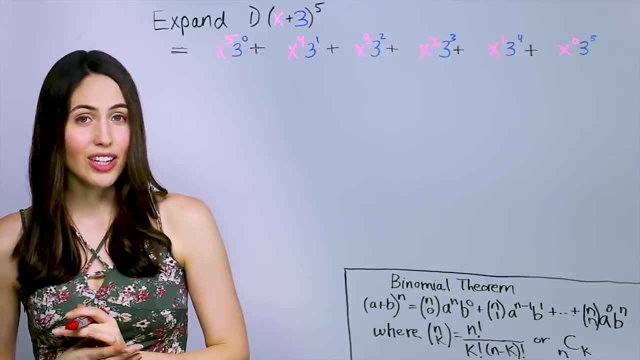 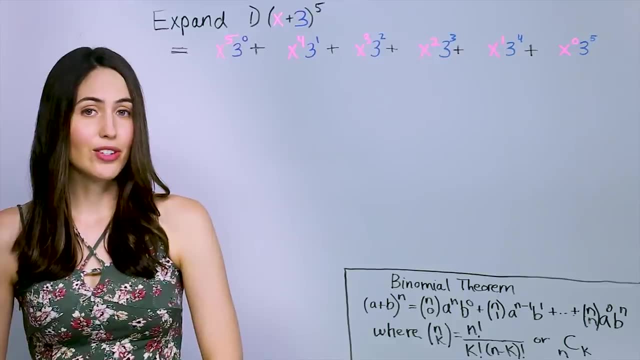 Okay, look, if you know about Pascal's triangle and that trick, good for you. It's very smart, very clever, and I'm going to use it in a minute, but first, really quickly, I want to show you the full theorem way. 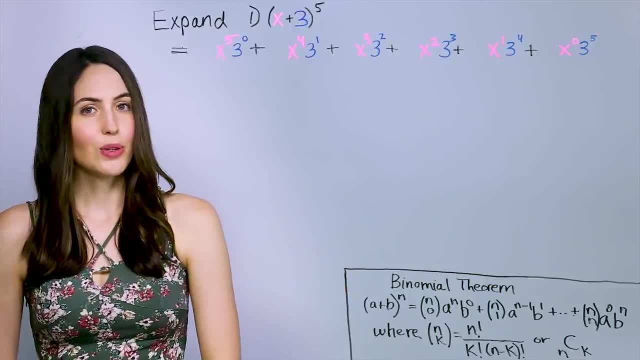 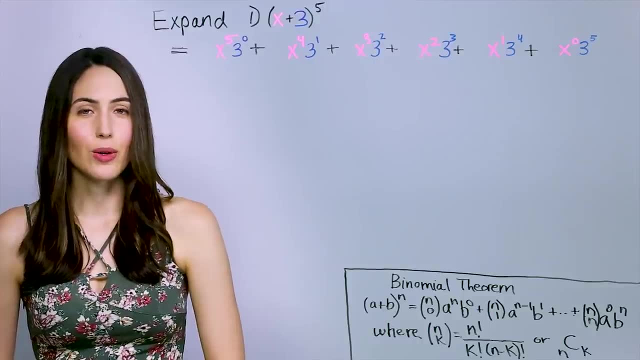 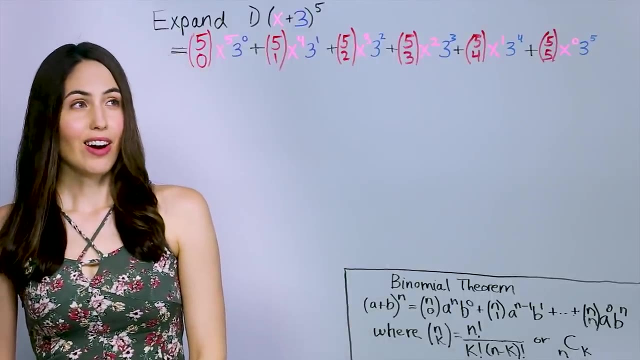 I want to show you the full theorem way of doing it, in case you need it, which you might. So let's do it that way. We're going to write the coefficients using something called combination notation. What are those? What is this five zero thing? 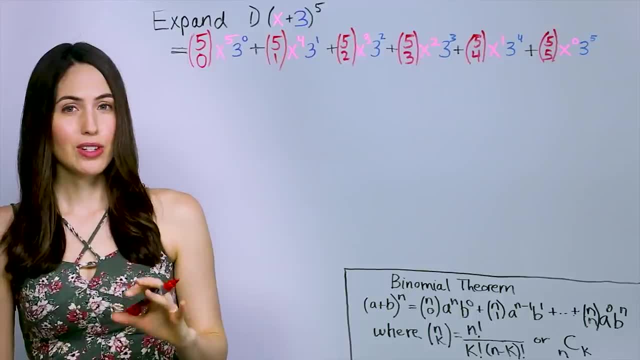 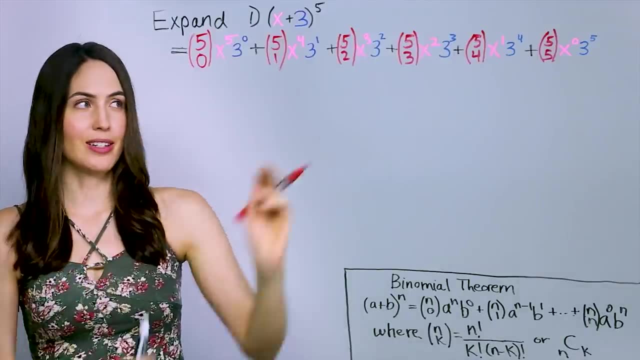 You might hear it said as: five choose zero or five choose one. Each of those is a combination of five, two and one. Each of those stands for some number that we're going to find, but when you're writing this out, the top number you write will just be your power number. 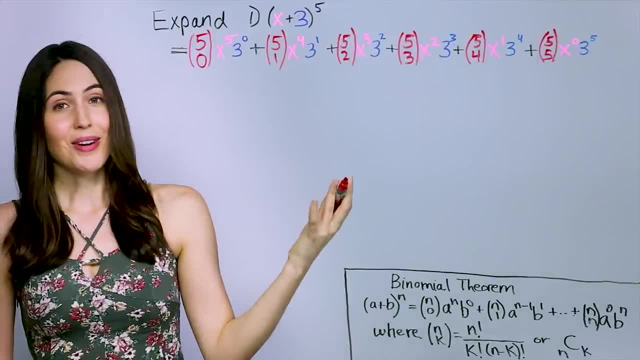 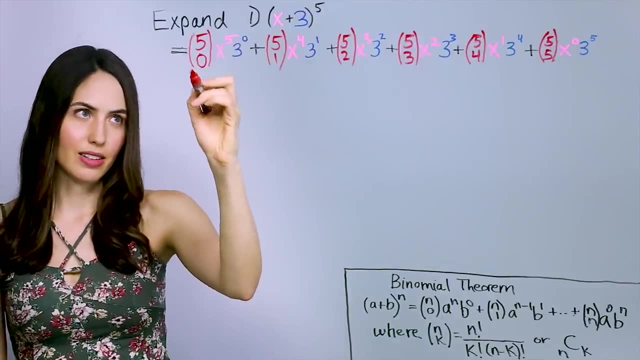 It's just five in all of these. It's also known as your n in a formula we're about to use and the bottom number when you're writing it just starts at zero and counts up. It's a counter all the way up to five. 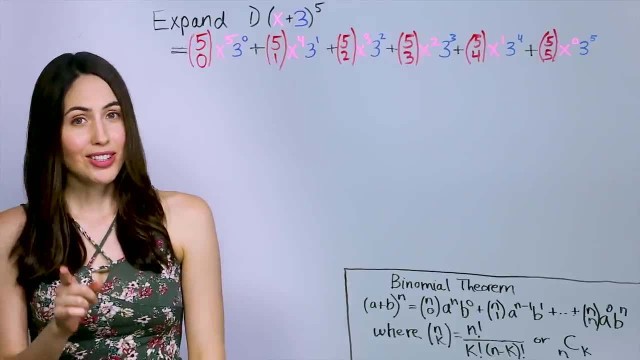 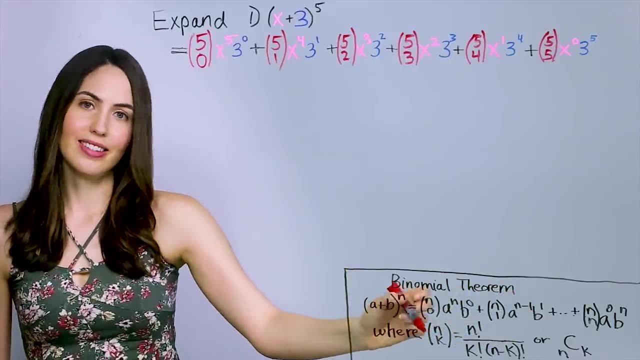 It's also known as your k down here, and if you just learned combinations, you might instead see this notation with a capital C instead of this. It's just notation. It'll give you the same numbers, But what does it all mean? 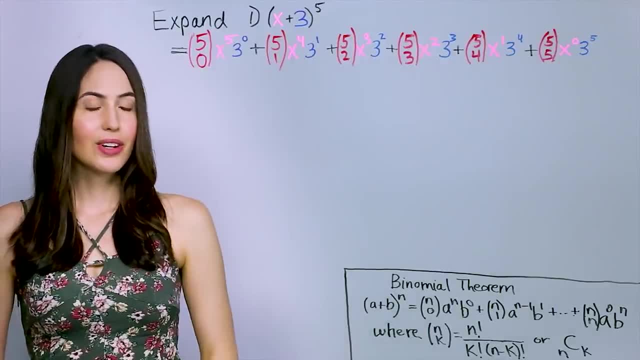 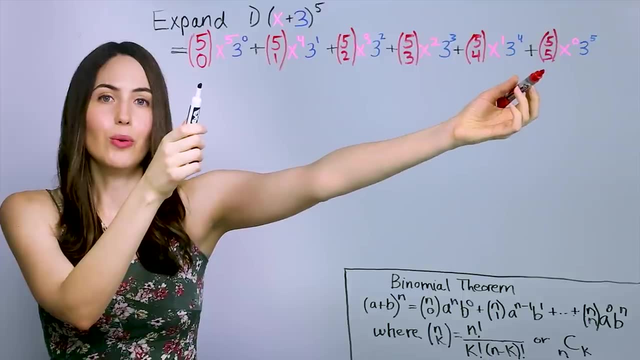 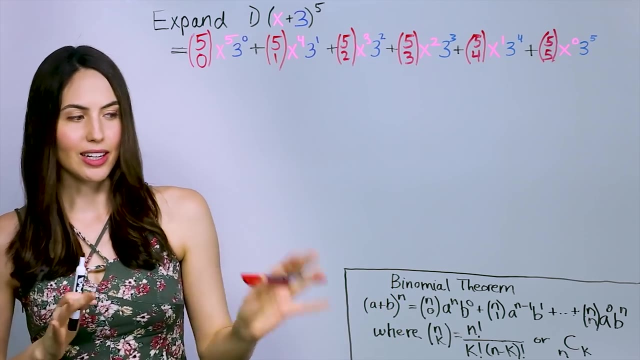 What do each of these really equal? First of all, to make your life a little easier. it turns out that the first one and the last one will always turn out to be one, even if you do use this formula, So you don't need to do the work of plugging. 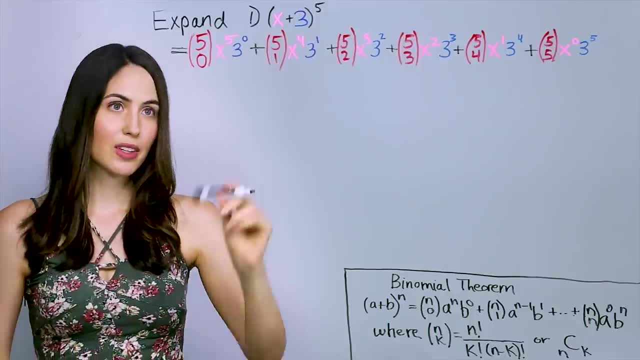 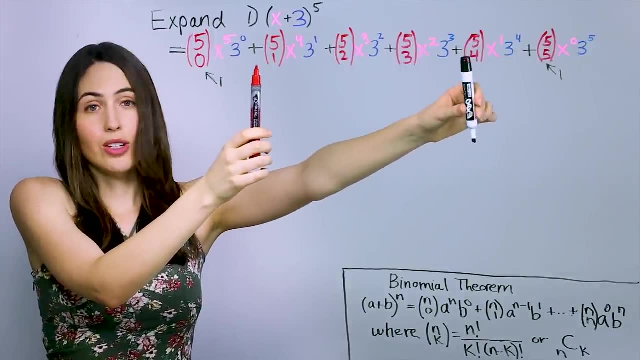 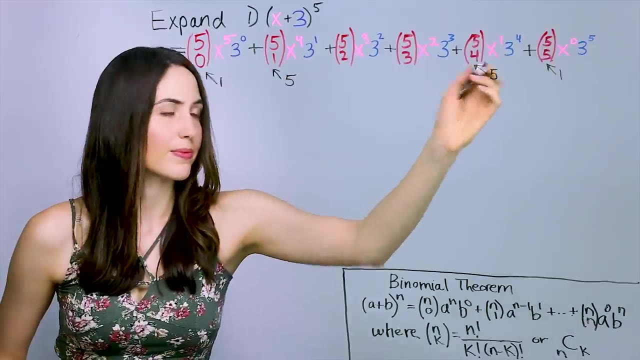 and chugging through that They're going to turn out to just be one Good news. The second number and second to last number will just be your power number five. They turn out to just be five. So just know that You can count on those things happening. 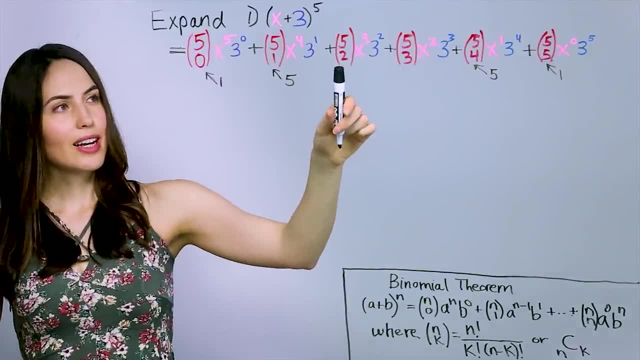 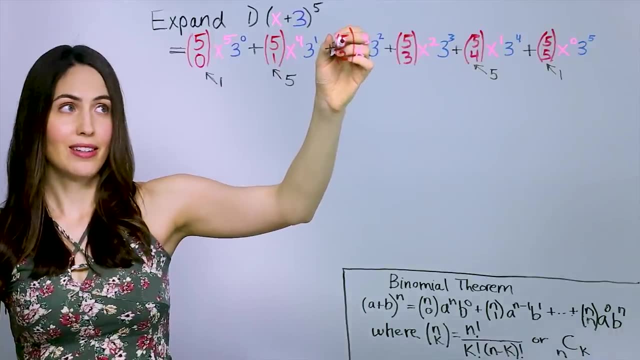 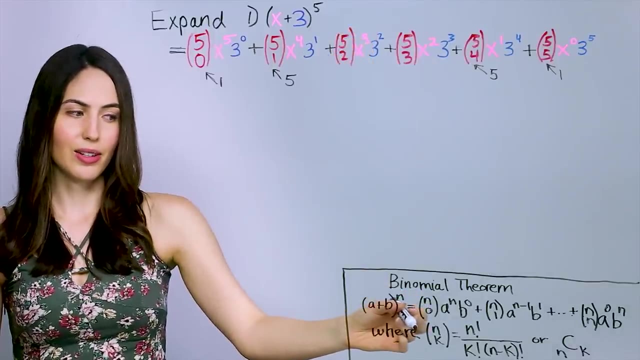 But what about this one, This next one? how do we get that? We will need to use the formula That top number is your n, Bottom number is your k. So n is five, k is two. n is five, k is two. 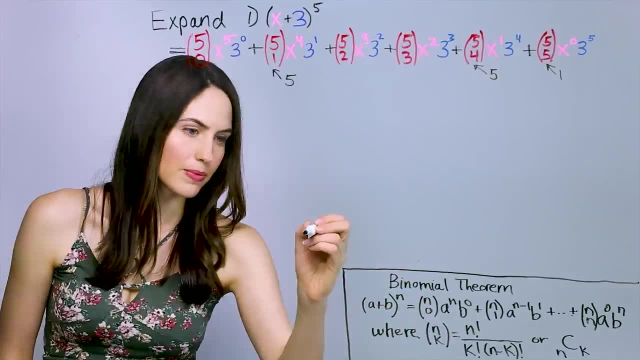 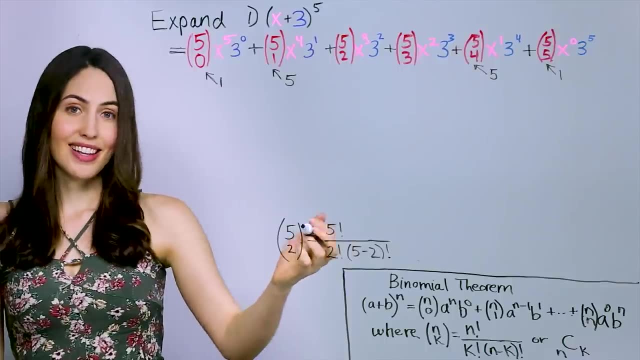 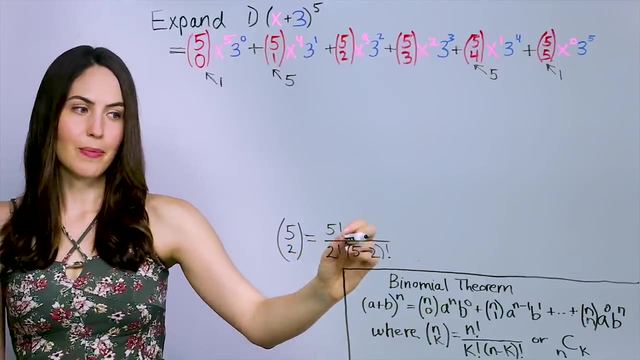 And we can just plug into this formula. Okay, so we can just plug into that equation. We have five factorial over k factorial, which is two factorial times five minus two factorial, And you can just simplify inside the parentheses. so that's good. 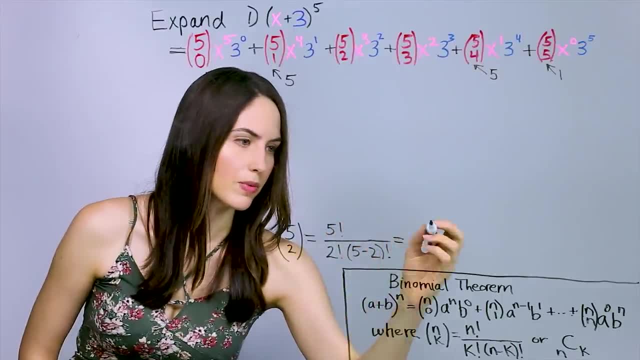 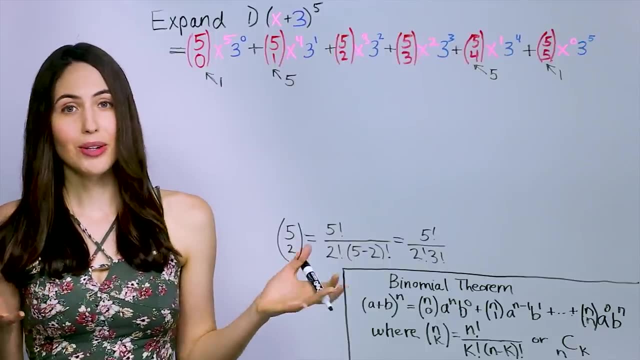 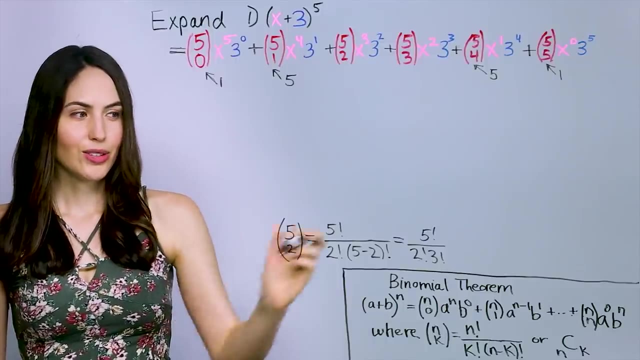 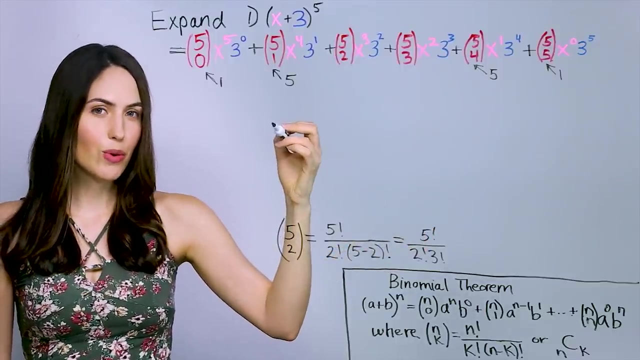 going to be three factorial like that. if you don't know or remember what the exclamation point factorial means, don't worry about it. it all it means is to multiply all the way down to one. so five. exclamation point five. factorial just means multiply five times, four times, three times, two times one, all of that. 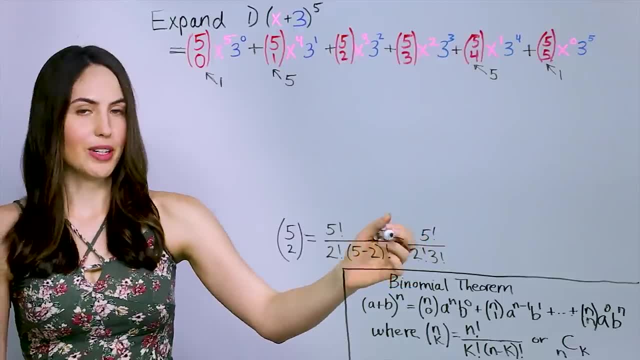 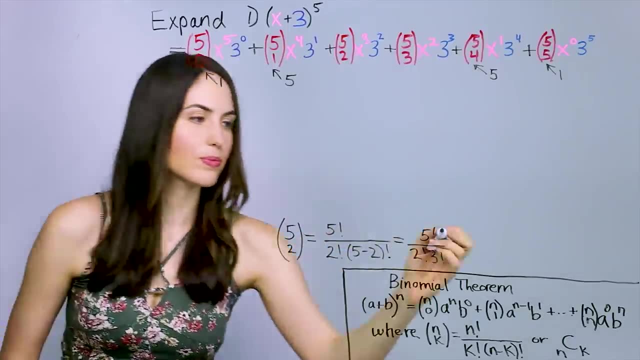 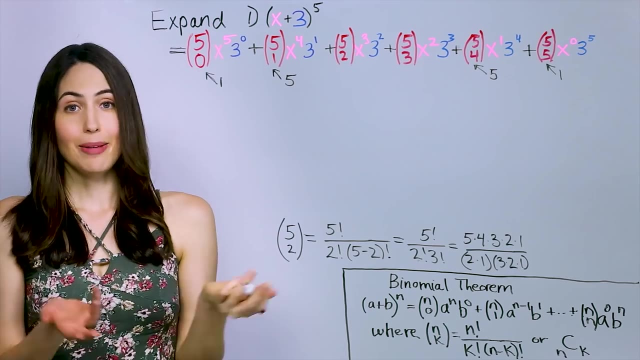 just multiply all the way down to one. so two factorial would just be two times one- that's it very short distance to go. and three factorial three times two times one. like that I'll multiply it out. and the benefit of writing it out like that is that you can see easily what will cancel, like the three times two. 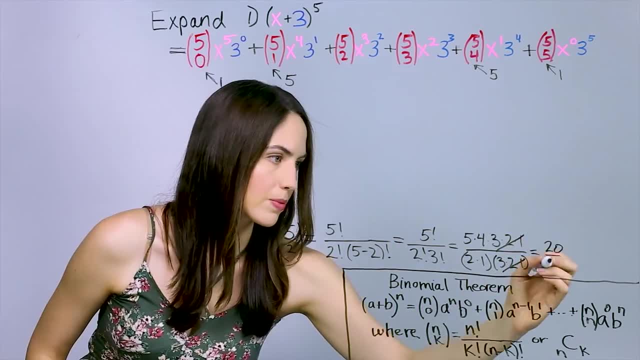 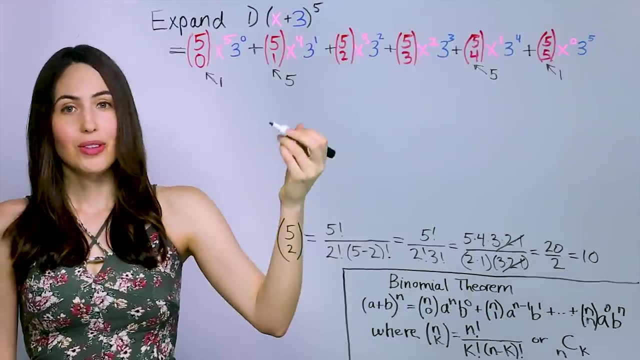 times one is the same on top and bottom- just cancels. and when you simplify it, you see that it's just ten. you see that it's just ten. you see that it's just ten. this whole thing just equals ten. so our coefficient there will be ten, great. 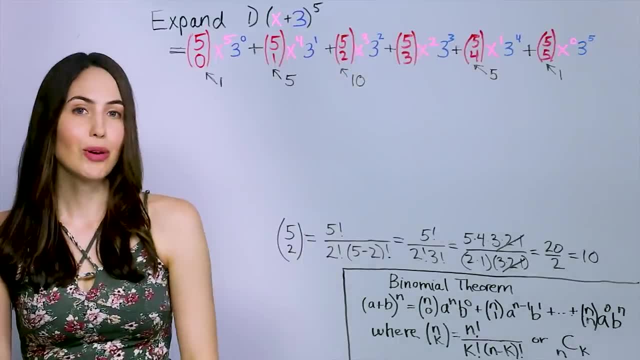 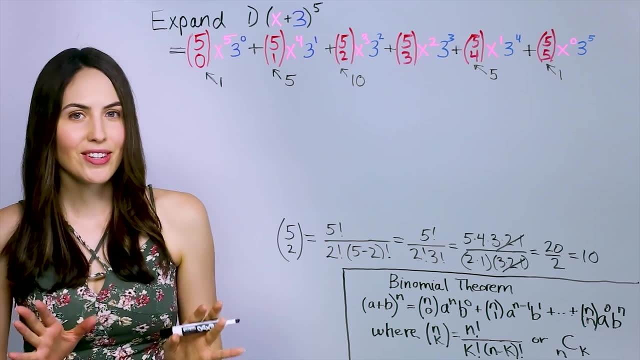 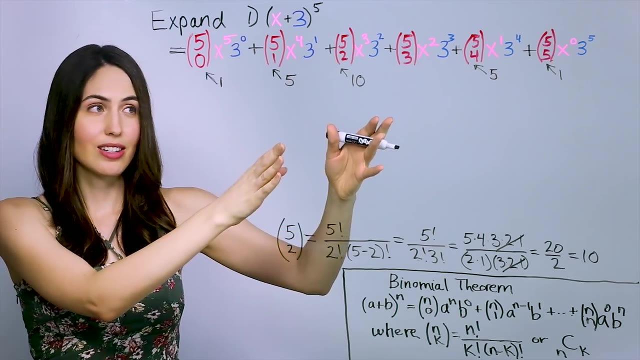 what about this last one? should we use that formula? yeah, I mean. yeah, use the formula. as long as you need it, it will work. but it turns out that in all of these coefficients for expansions they are symmetric, so they're the same forwards and backwards. so you can tell. if it was already. 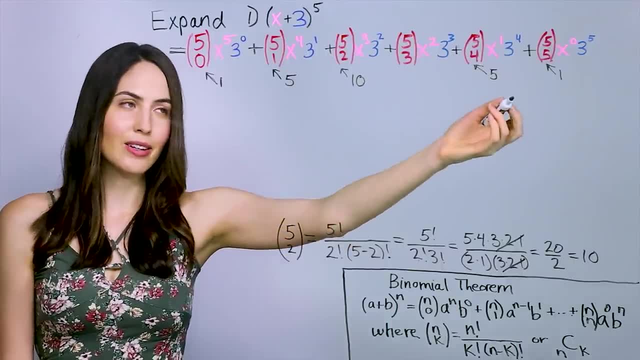 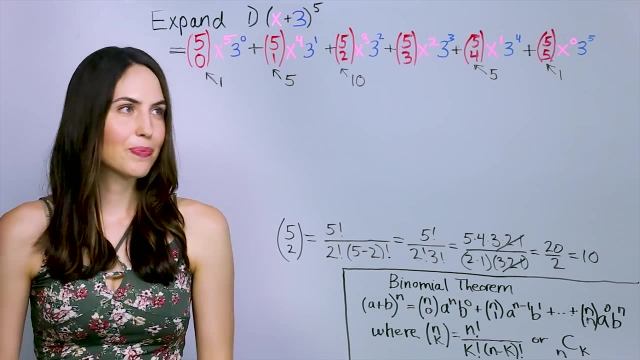 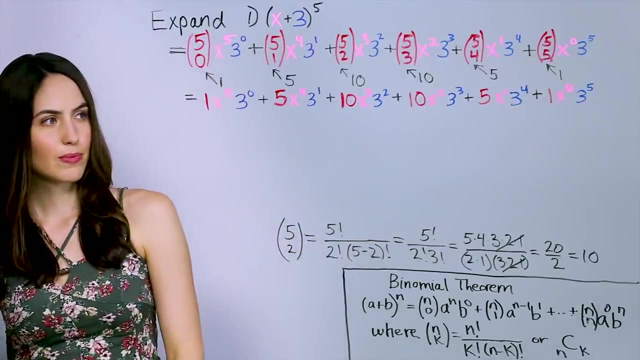 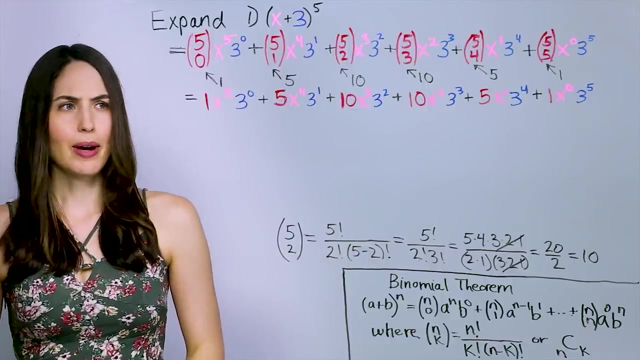 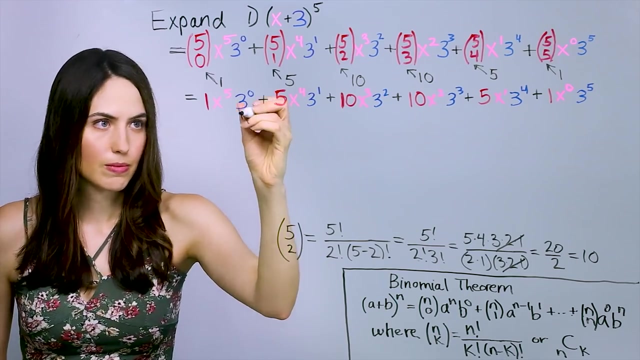 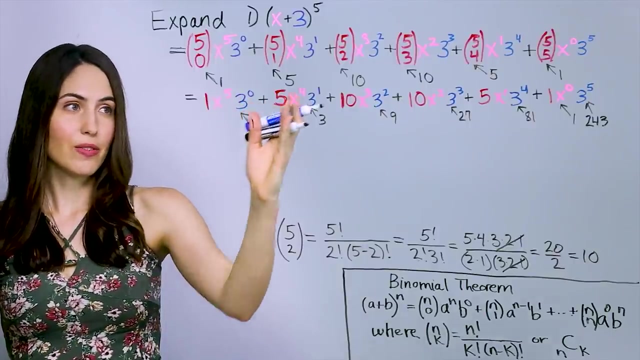 going to be one five. feel about that. that did not work. but when you do one, five, ten, something, five, one, this is gonna have to be 10 because for it to be symmetric mirror image, so we to the zero, Those are just one, And also we can just write what these powers of three. 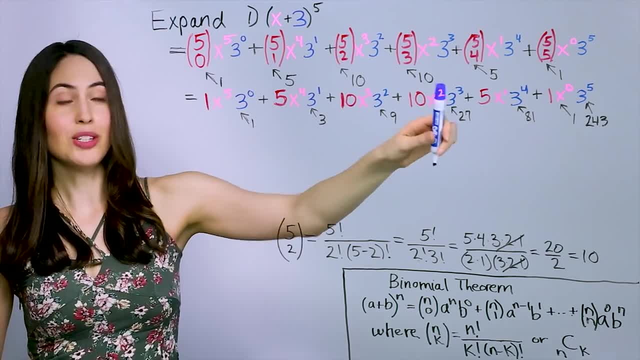 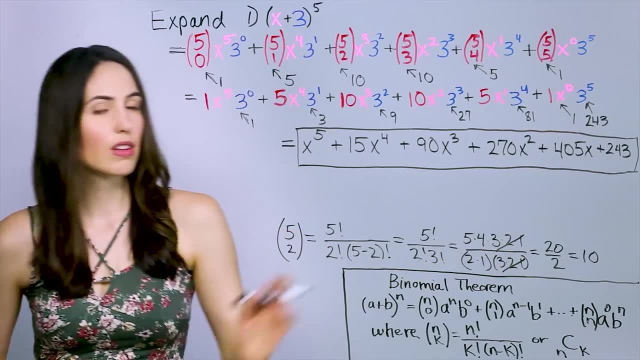 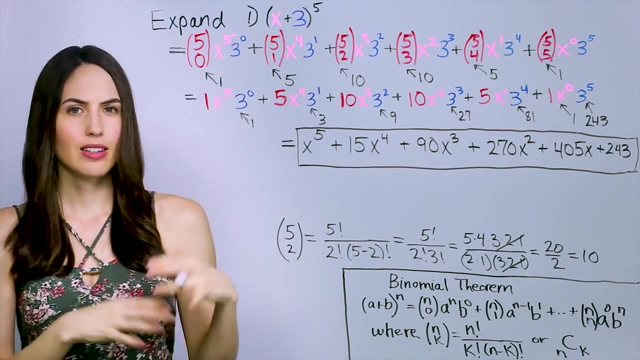 really are like 3, 9,, 27,, 81,, 243.. So that's it. That's the answer, And you don't need to write these ones. when you're multiplying by ones, by the way, It doesn't matter in. 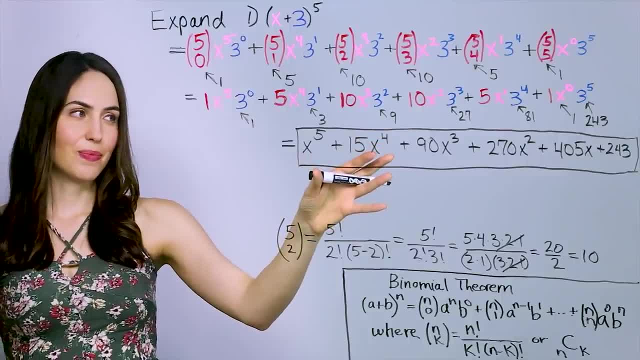 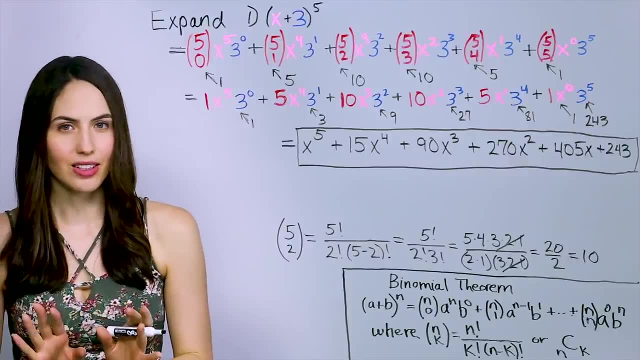 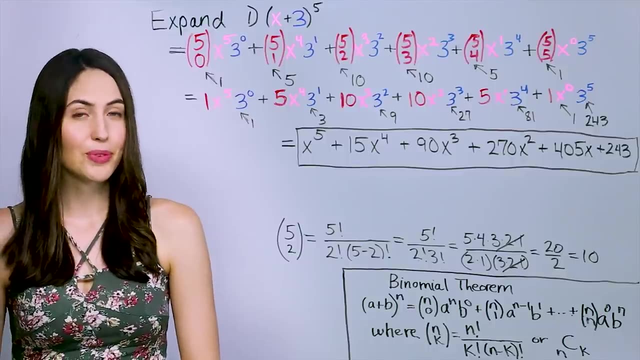 the end. This is the simplified answer. This is your expansion. Good times, Good times. I know this took a long time. It's just because it's the first one, But when you've done this a few times, it's going to be really easy for you, Really. By the way, there's a button. 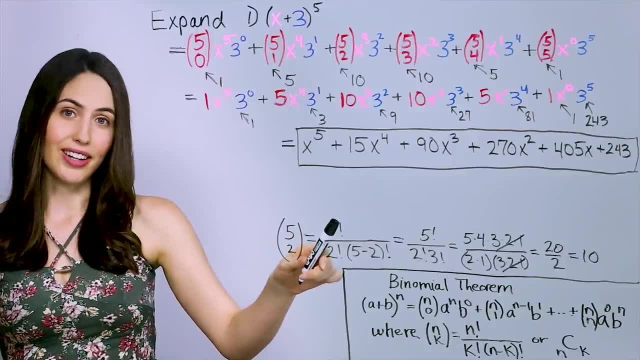 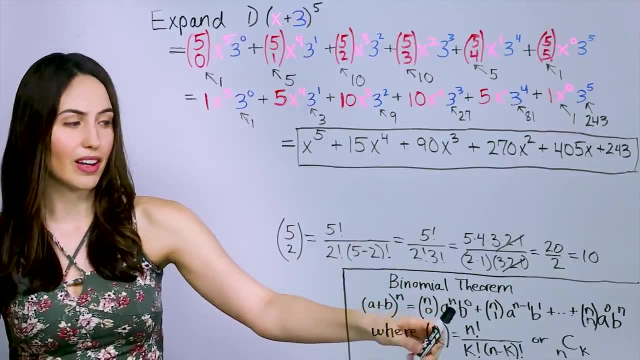 on your calculator for n factorial. if you want to use that- And, even better, there's a button on your calculator for this- I'll give you that. I'll give you the number for that. It's usually listed with this notation, So it actually. 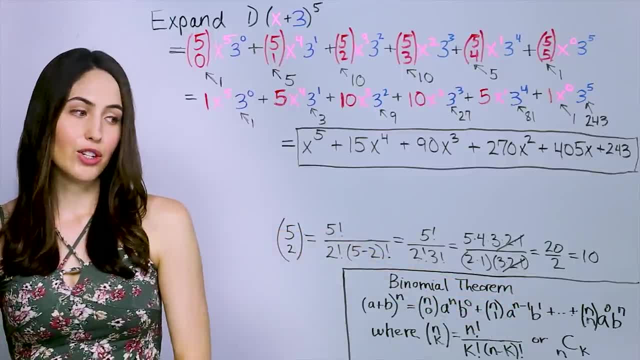 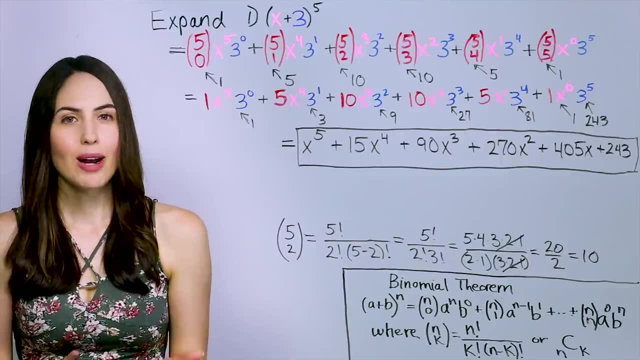 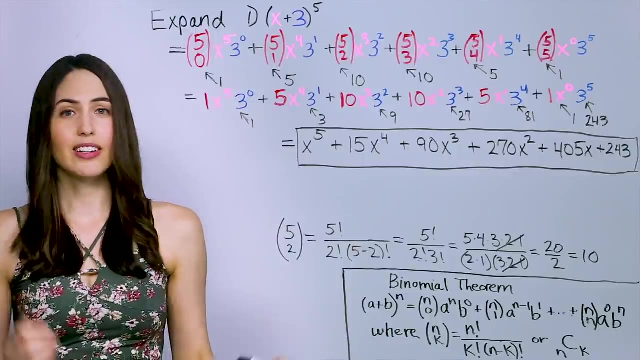 usually says ncr, But you can use that to get these numbers If you don't want to do it by hand. it is faster, All right. What about Pascal's triangle? This is really complicated, you say, And couldn't we have just used Pascal's triangle? Yeah, Pascal's triangle can be a. 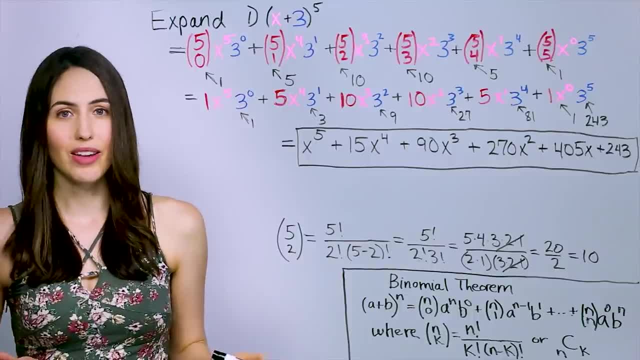 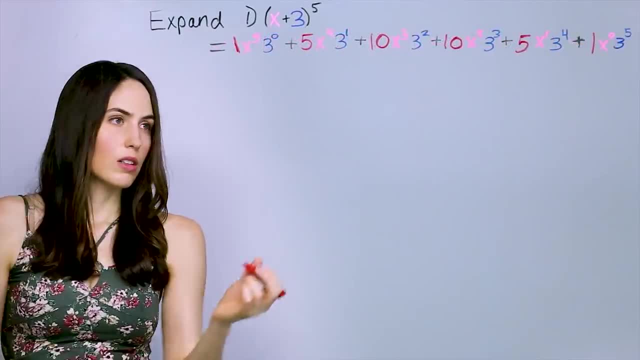 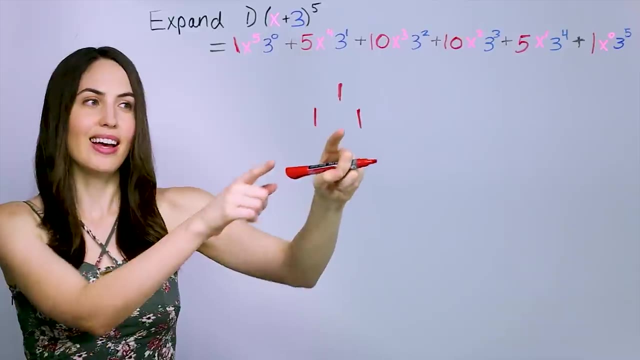 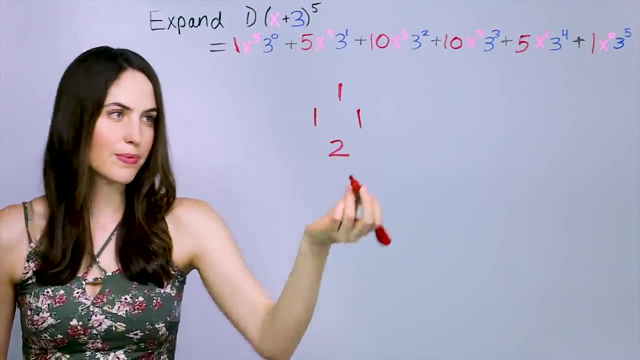 really easy way to just grab all those numbers at once and be done with it. Start by drawing three ones in a little triangle And then underneath get another row of numbers by adding the two numbers above, So one and one will give us two, And then. 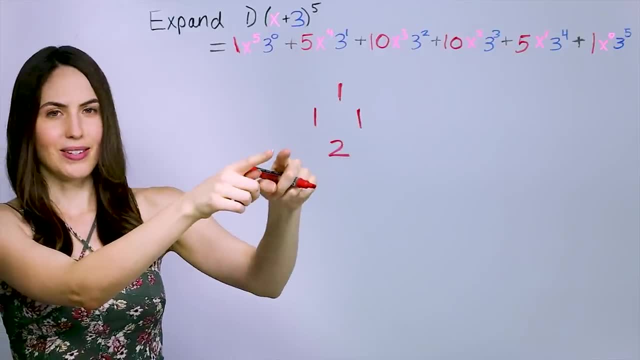 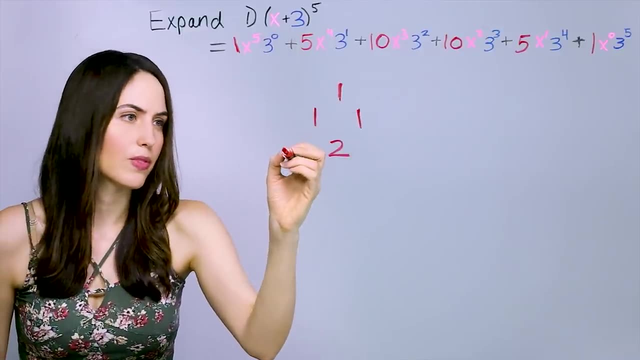 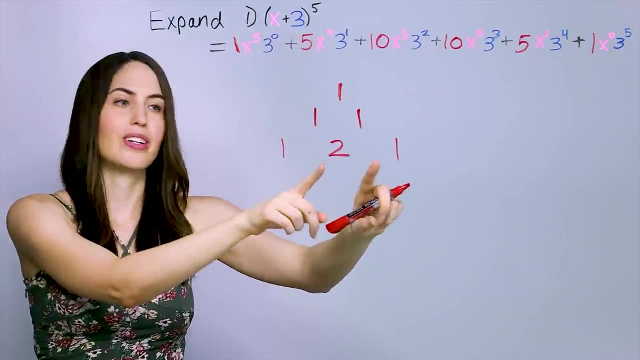 on the outsides, just carry down the ones. So here, since they're not two numbers above, there's just the one. Just carry down the ones on the edges And then, if you keep going, adding the two numbers above, so one and two will be three. 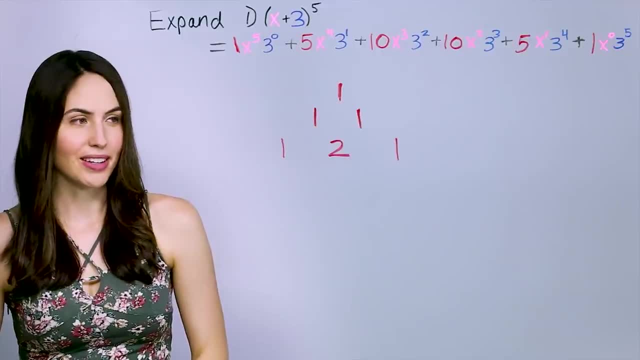 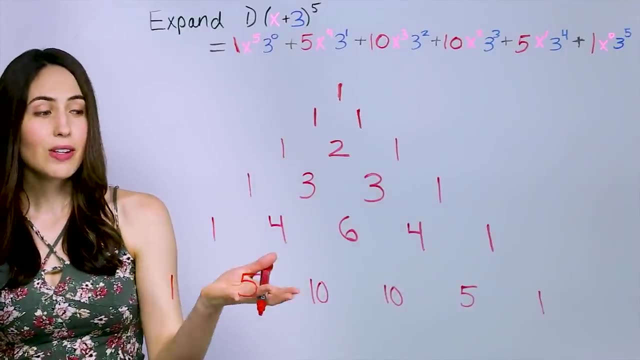 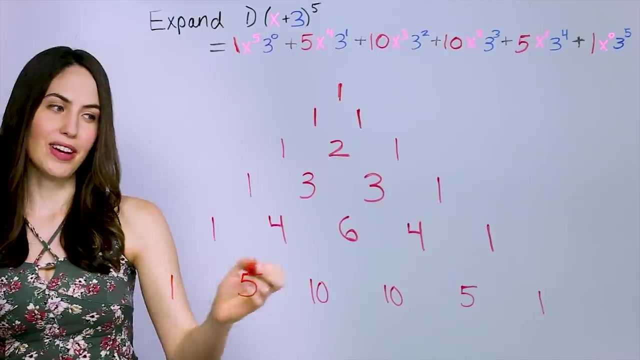 Two and one will be three If you keep going. it will give you exactly the numbers that you need, Exactly the coefficients you're looking for in your expansion. So one, five, ten, ten, five, one. That was our one, five, ten, ten, five, one. 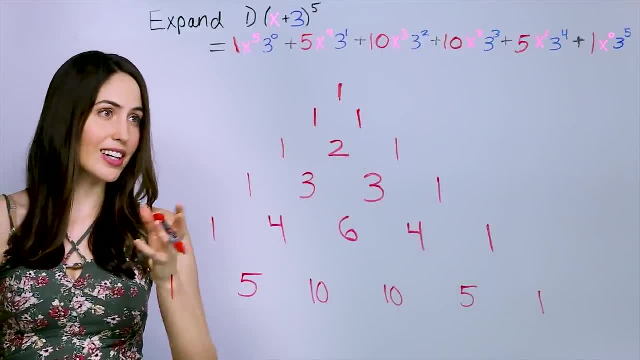 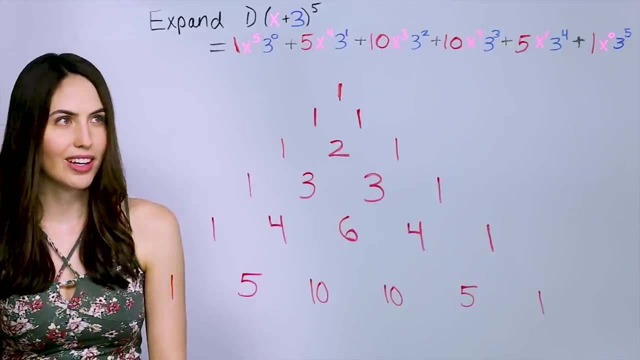 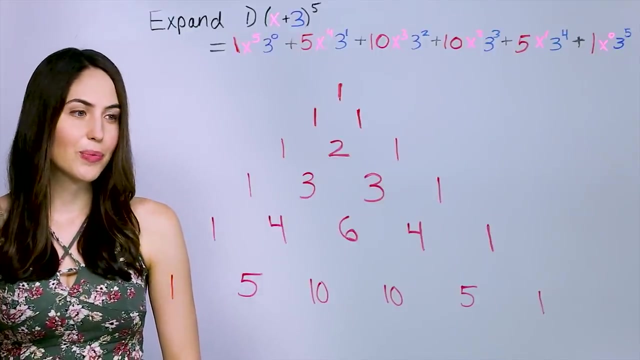 like magic. What is this mysterious triangle? Kind of dark magic or secret Illuminati pyramid? It's just Pascal's triangle and as long as you're willing to write out the rows of the triangle, it will give you the numbers you need for your expansion. So whichever row of the triangle has your power number in it, as 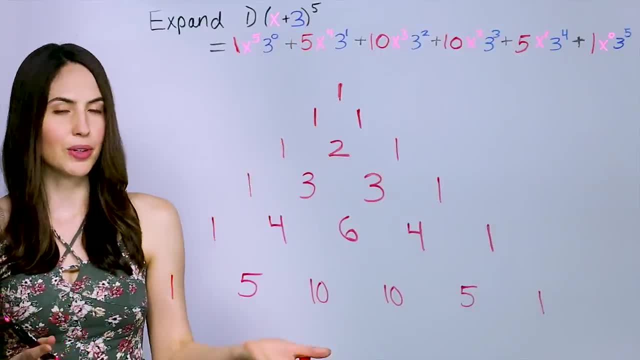 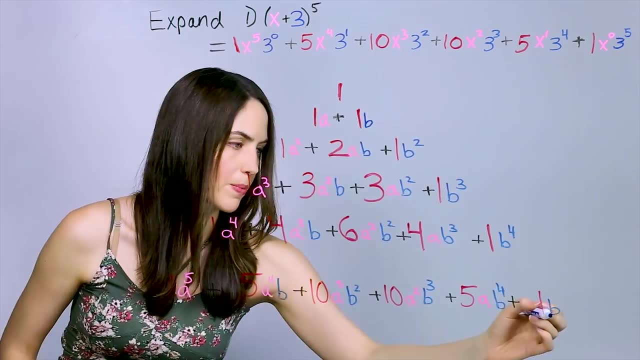 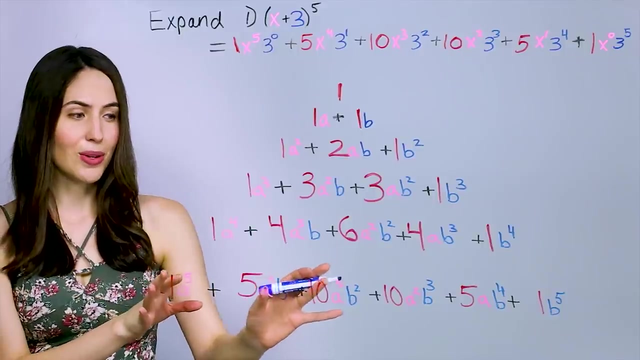 the second number is the one that will give you the numbers you need. Okay, so you don't need to write the variables I just wrote. I'm just doing it to show you how those numbers go. with an expansion Like this is a plus b to the. 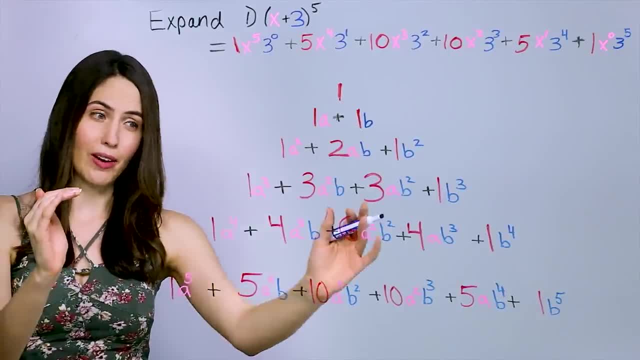 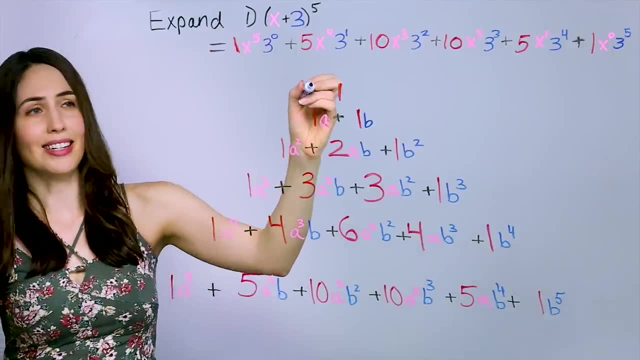 fifth power, That's the whole expansion, a plus b to the fourth power, has those coefficient numbers. The third power, this row's second power, first power, zero power. This is technically row zero of Pascal's triangle. Row one, two, three, four. 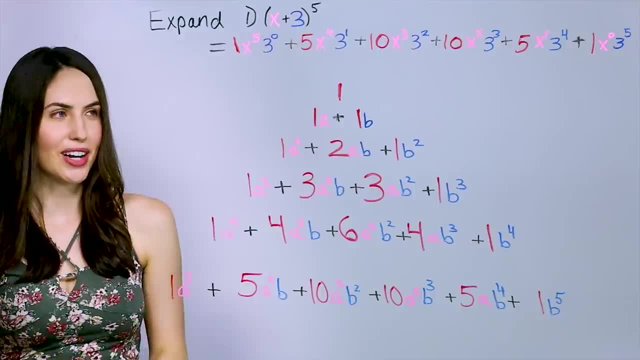 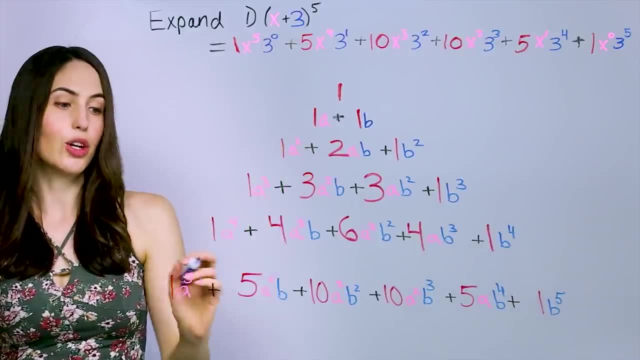 five. We're doing a lot of counting from zero here. That's a theme, So all you need to do, though, to use Pascal's triangle, is write it out. One, one, one, one, two, one, Grab the numbers you need, plug them in as coefficients, and from there it's the. 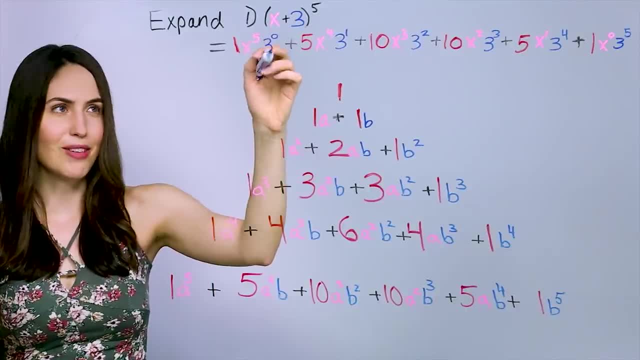 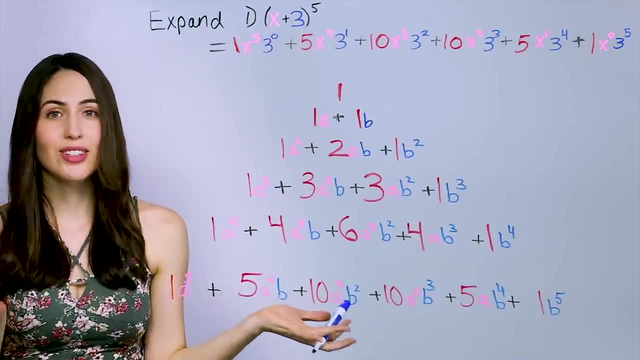 same as before, Like the powers, and the pattern of powers is the same. Simplifying is the same, So that's all you have to do. So why don't we just use Pascal's triangle all the time? right, It's a good question. 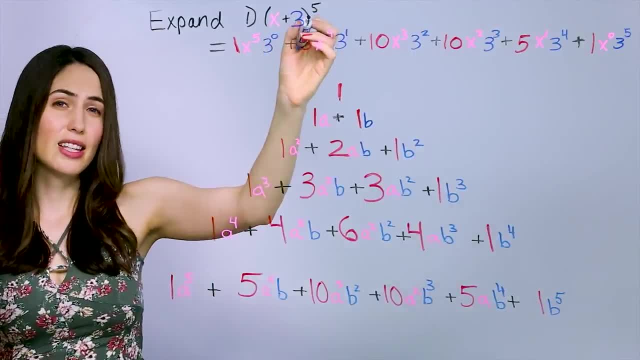 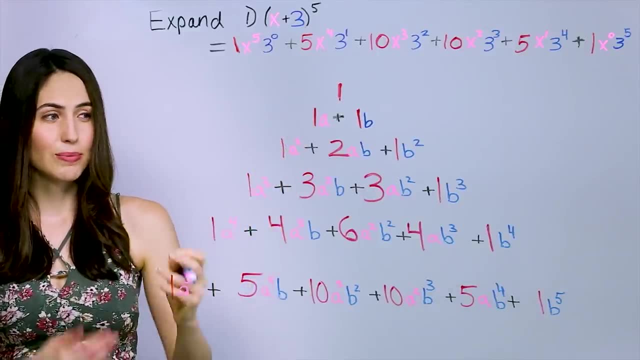 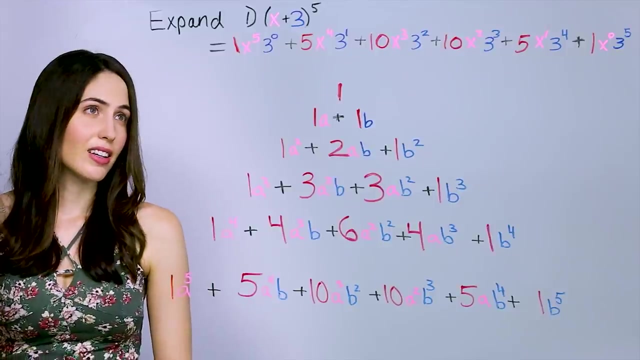 I mean, if you got something like the 15th power, maybe you're not gonna want to write out all 16 rows of the triangle like the ever-expanding triangle. Suddenly, Pascal's triangle may not look so cute anymore, But you have a choice, You can. 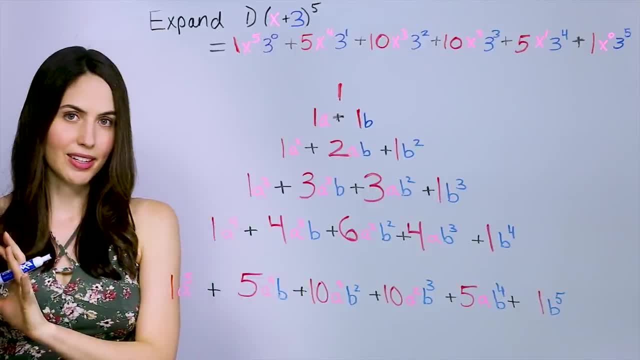 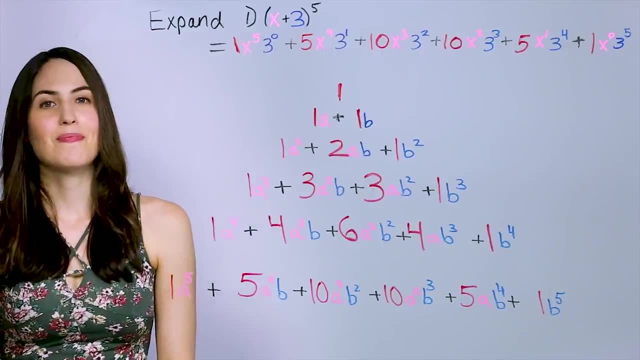 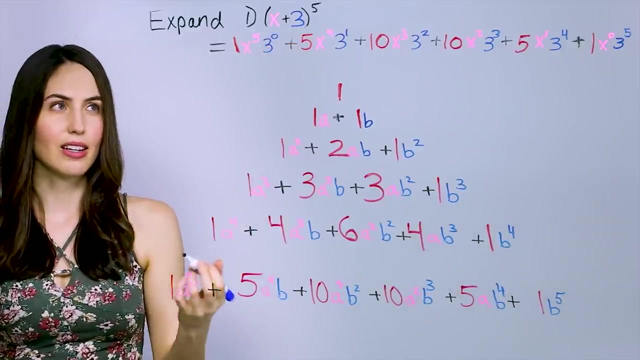 use the triangle or the formula combination formula with NK, Either one will give you the same numbers. Now how do you do an expansion if you have subtraction instead, Like a minus b, A difference, How would you do it? And how do you do it if you have a number on the 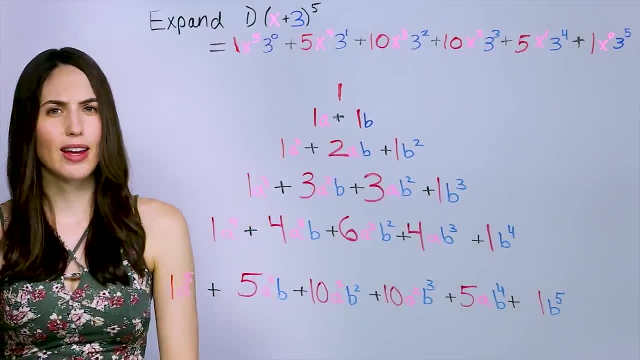 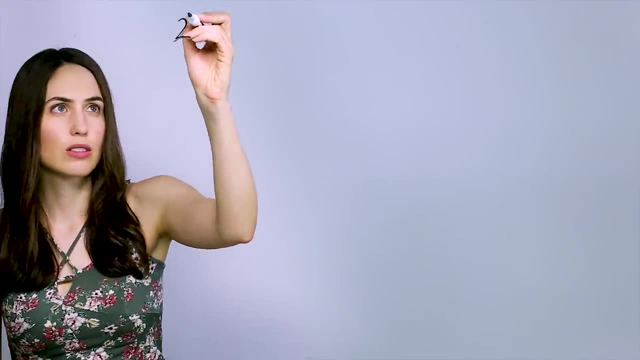 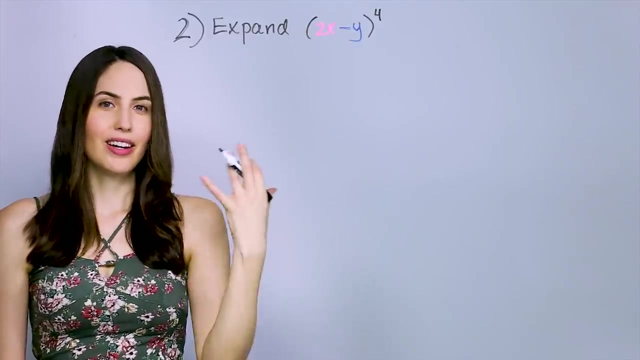 coefficient like 2x instead of x. What then? It's basically the same idea. Let me show you. Okay, so we have 2x minus y, raised to the fourth power, A difference kind. It's gonna be the same idea as before. It's just that for the 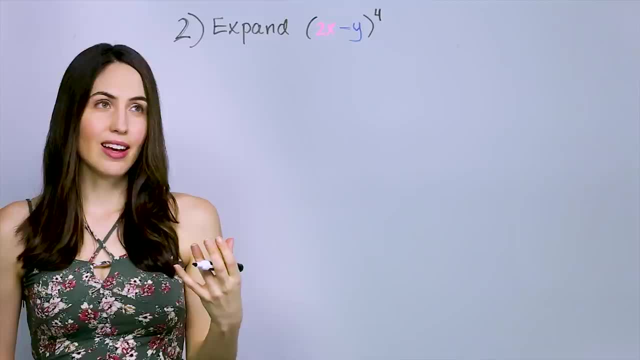 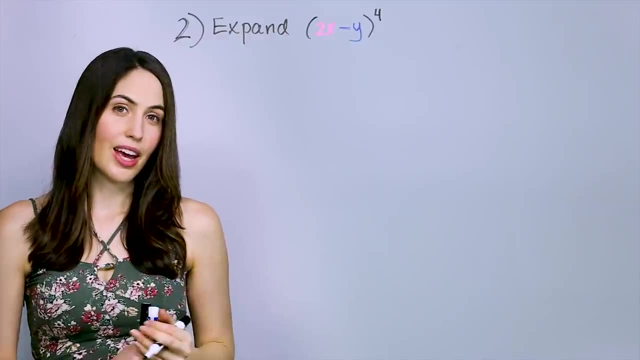 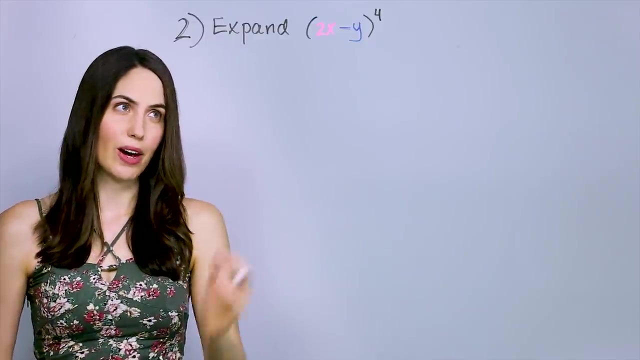 subtracted part minus y. think of it as a negative y being added like plus negative y, And then all of negative y will get raised to a power, All of negative y- in parentheses- raised to each power. So you might have already guessed. 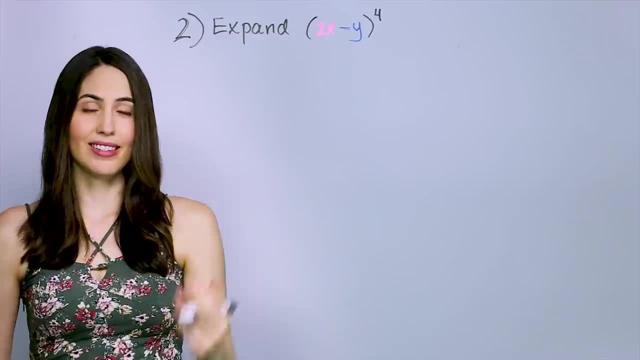 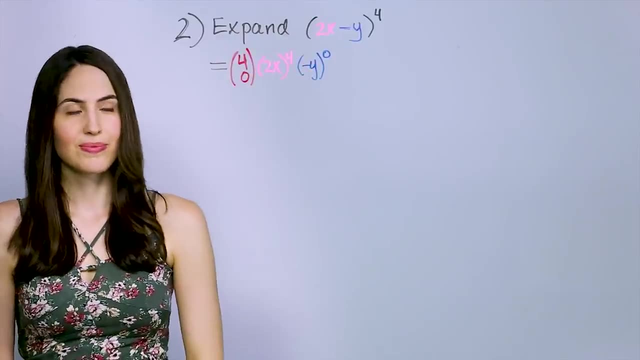 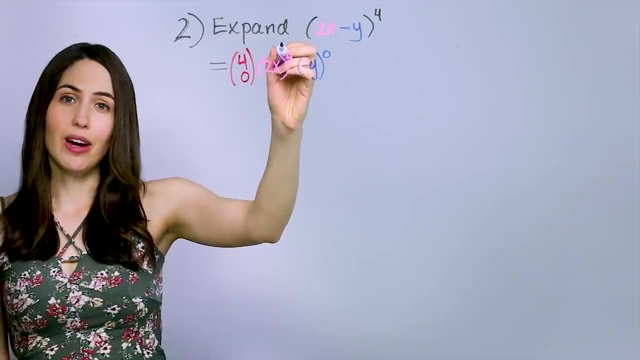 it, but for the 2x, the way you handle that is that all of 2x- in parentheses- will get raised to each power. So you see, for the first term, this first factor, all of 2x, starts at the highest power and it's gonna go down by one. 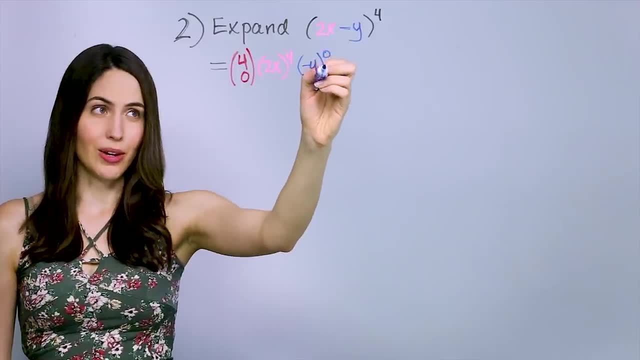 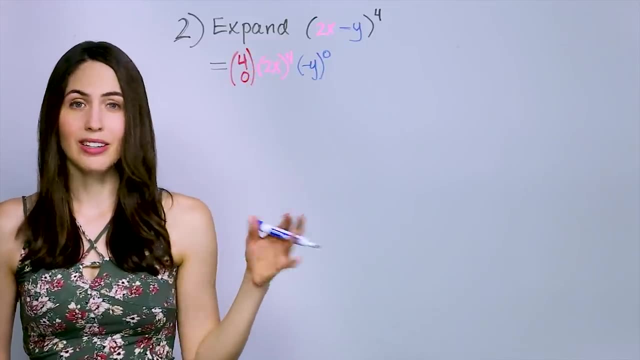 And then the second power negative y- all in parentheses- starts low at the zero power and will go up And we have this: 4 choose 0. And we can write the rest of it. now We don't even need to look at the binomial theorem. 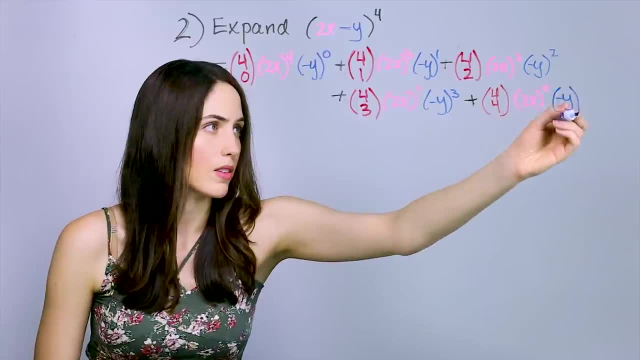 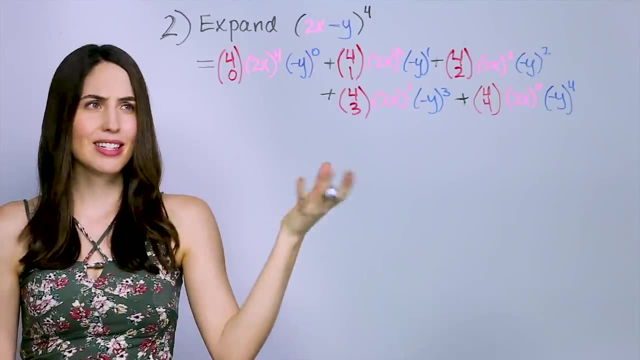 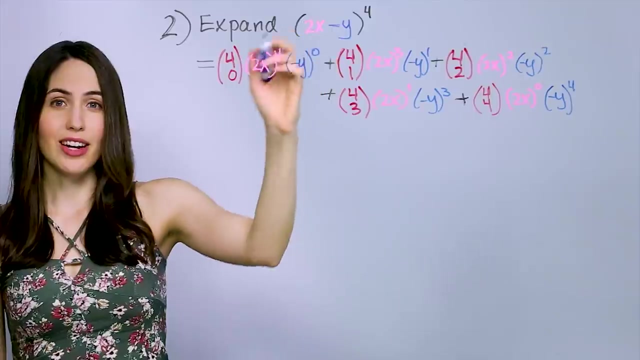 So that's it, that's the expansion. It's not so bad right, It's the same idea as before. Those coefficients, you know how to get those 4, 0,, 4,, 1,, 4,, 2, etc. First factor gets. 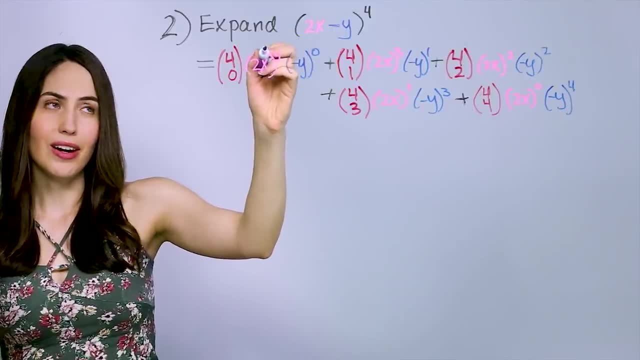 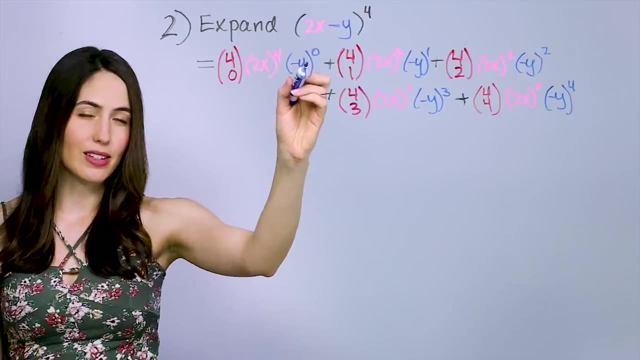 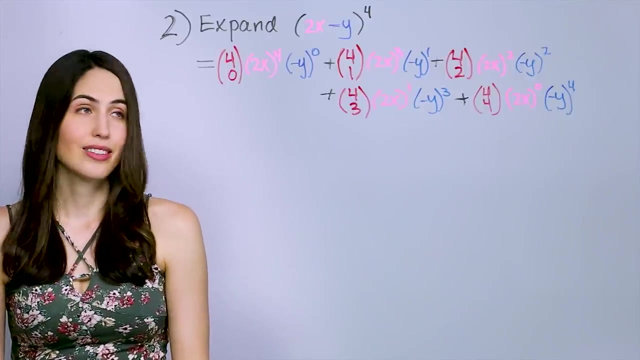 raised to the highest number- power, our power number- and then goes down each term. Second factor: gets raised to lowest zero And then increases 0. 0. 0. 0. on each term. You just need to simplify it. Be careful, The place where a lot of people trip up. 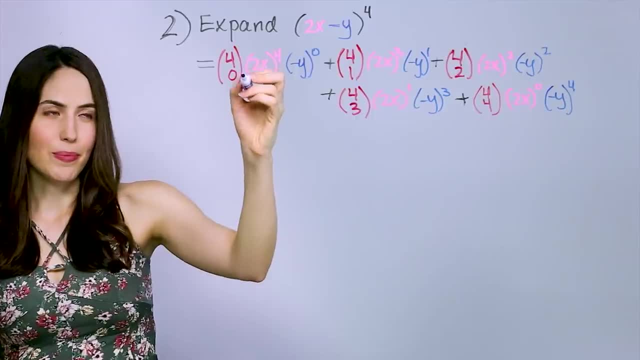 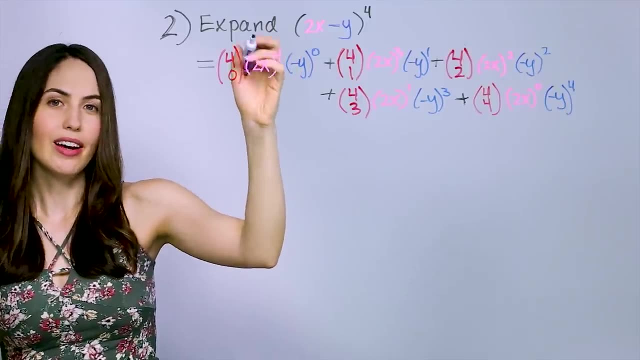 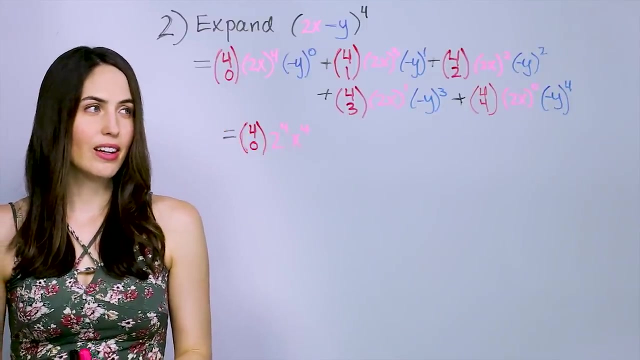 is simplifying something like this, Just remember: the 2 gets raised to the power and the x gets raised to the power, each of them. So 2 to the 4th power, x to the 4th power, And then for these negative y's- to simplify anything- to the 0 power. you know is just going. 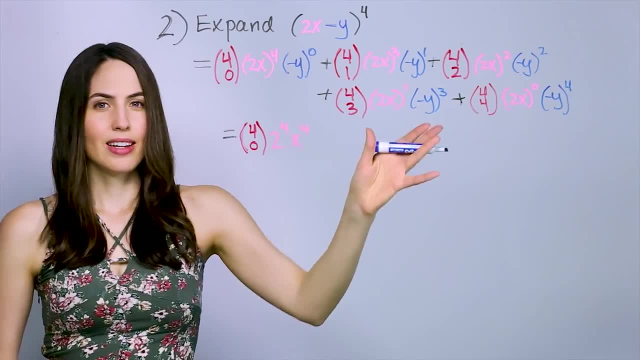 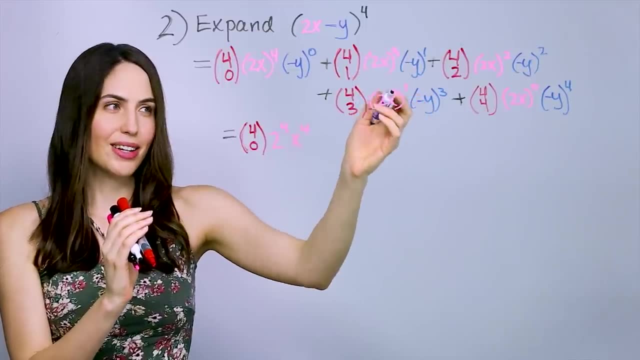 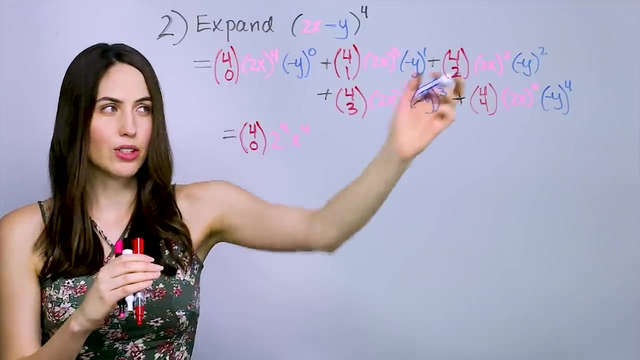 to be 1.. But what about these negative y's? Yeah, just remember. so negative y raised to an odd power, like 1 or 3, will stay negative overall, And negative y raised to an even power, like 2 or 4, will become positive overall. 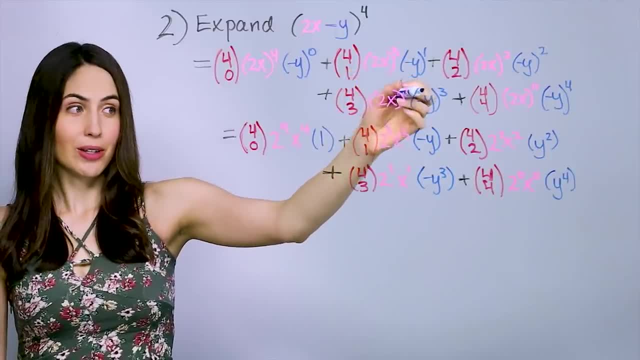 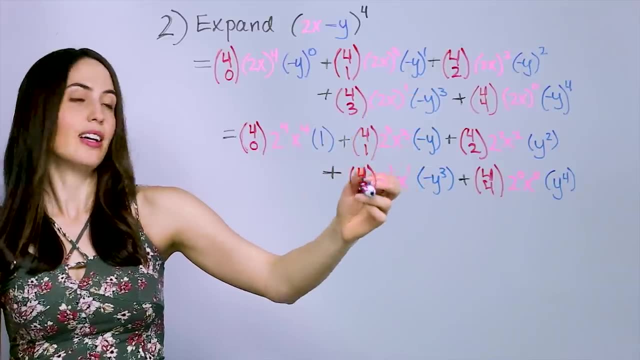 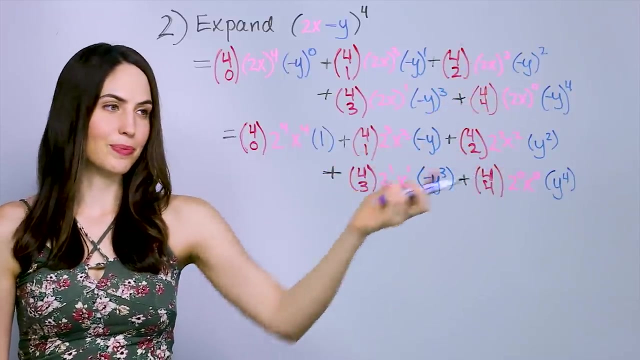 So negative y's to the odd powers became negative overall. So negative y to the 1st power is still negative y. Negative y to the 3rd power is overall negative y cubed. And then these 2 became positive overall. So now we can just write. 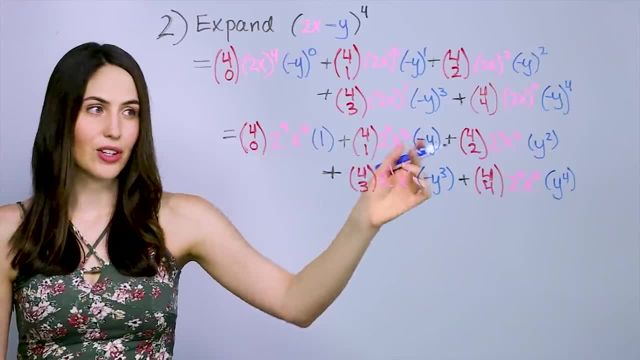 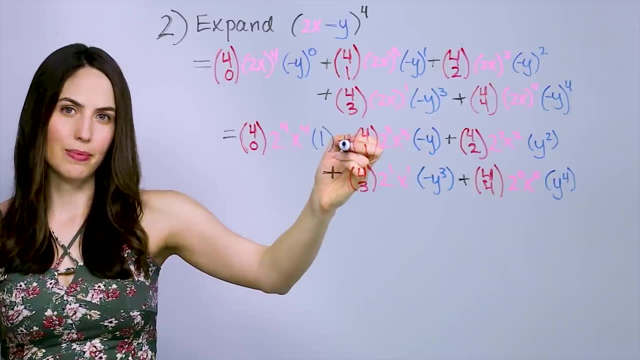 what those powers of 2 actually are, 16,, 8,, etc. And any negative you have, you can pull the front of the term And adding that negative. you can pull the front of the term And adding that negative. 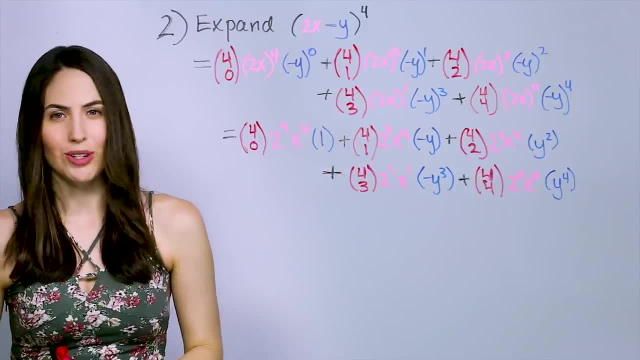 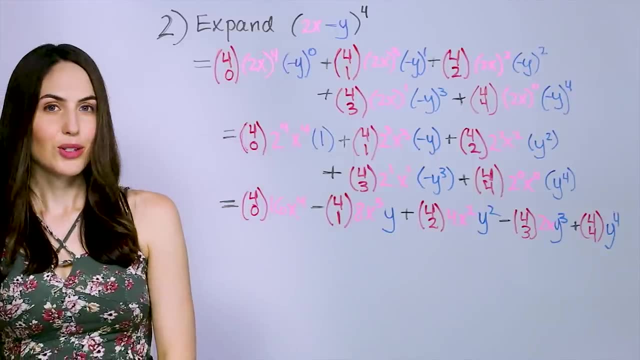 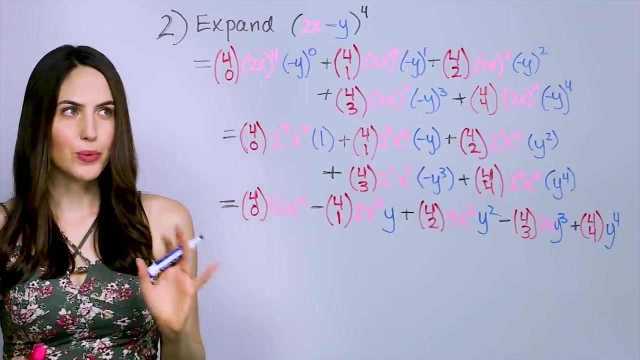 basically becomes subtraction of the whole term, So you can just write it that way. So notice how the sign keeps switching: Positive, negative, positive, negative, positive Switches like that. That's what happens in this difference kind of expansion. Now we just need to find out. 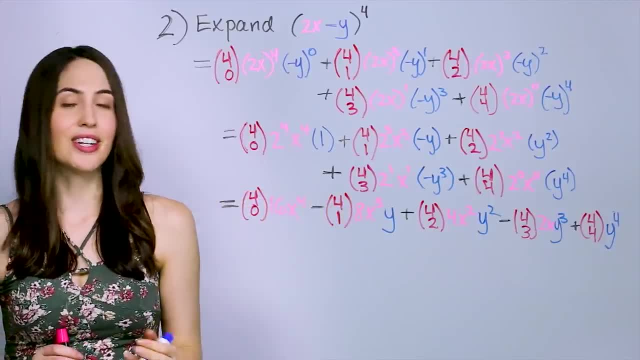 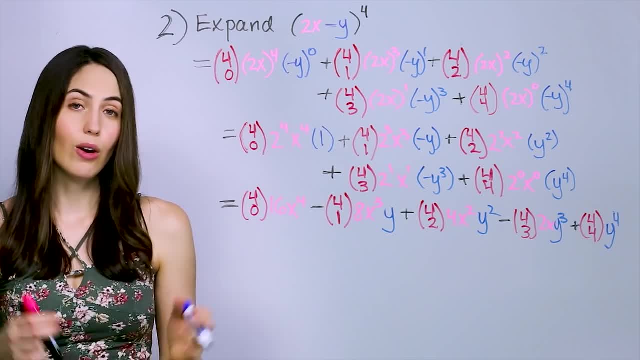 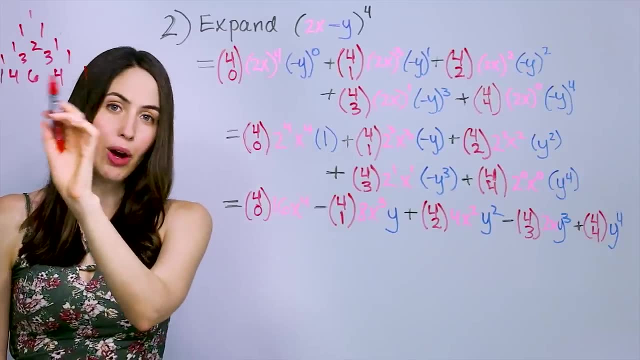 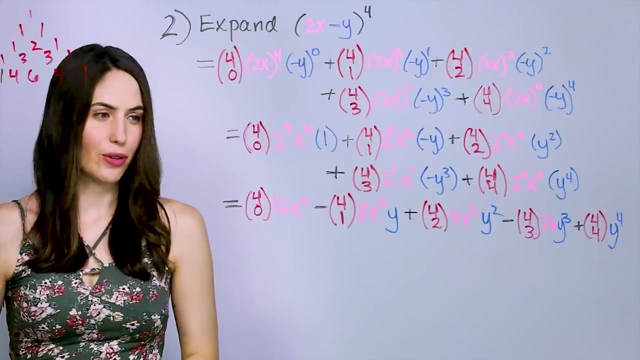 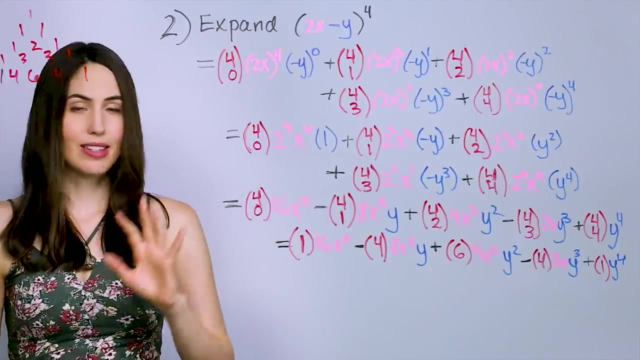 The combination formula button on your calculator, or Pascal's triangle, Mini Pascal's triangle, But you just want to grab whatever row has your power number in it. The second number, This one, 14641.. Those are coefficients. Clean it up a little, Simplify a little more. 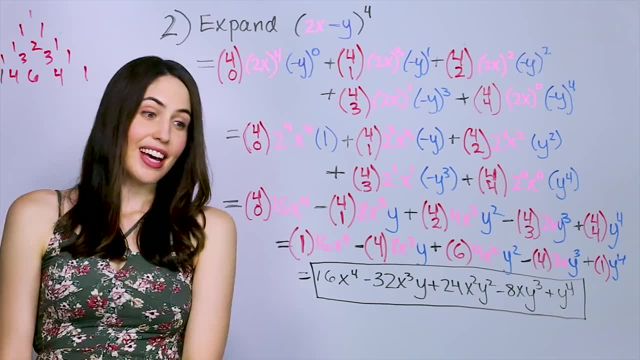 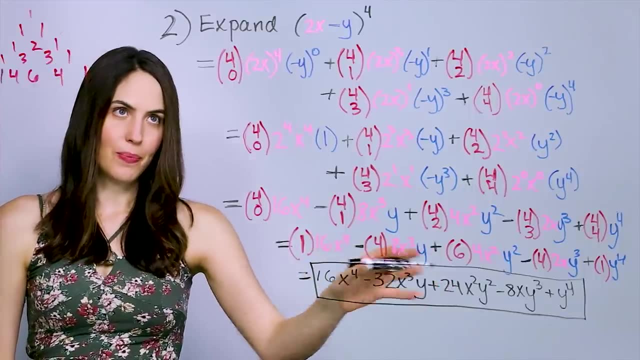 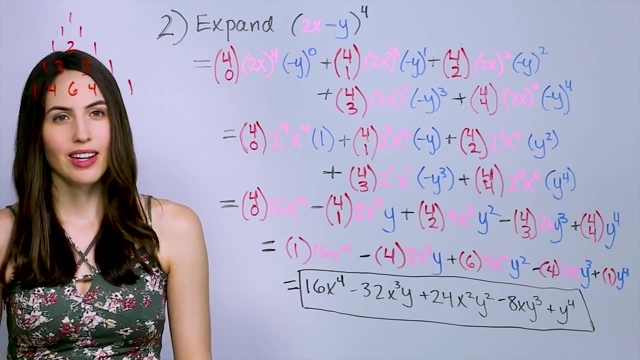 And that's your expansion. Yeah, so the sign does keep switching, flipping between positive, negative, positive, negative. It alternates between the two. So that's it. That's how you do binomial expansions. Just a few miscellaneous, random. 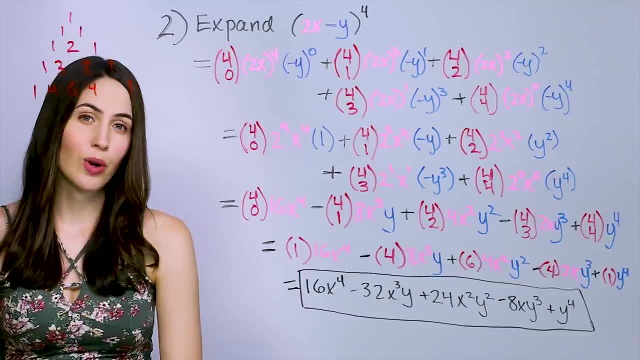 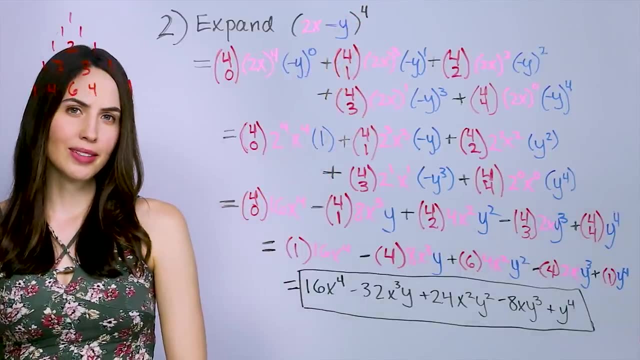 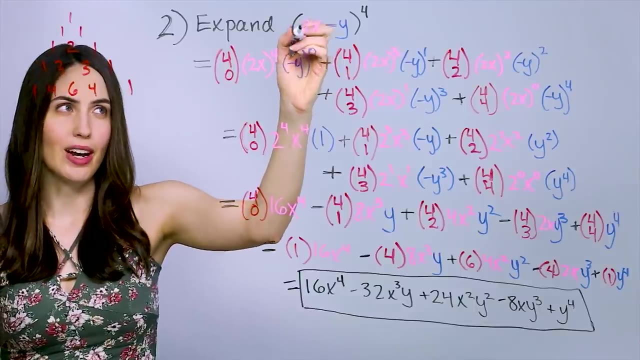 things. The binomial theorem doesn't work for fractional powers like a fraction power like a one half, In case you were wondering, which many people do. it's fine if you have a fraction inside the binomial as a term: one half plus x, one half minus y. That would work Also, the binomial theorem. 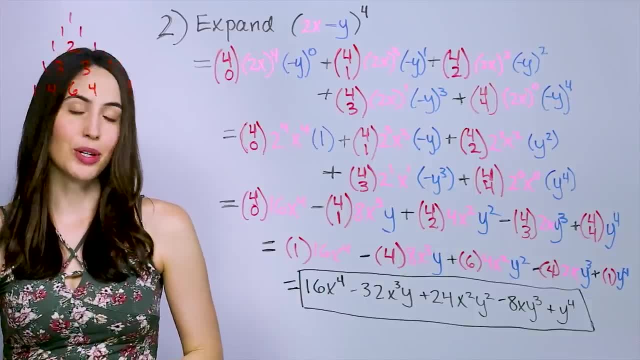 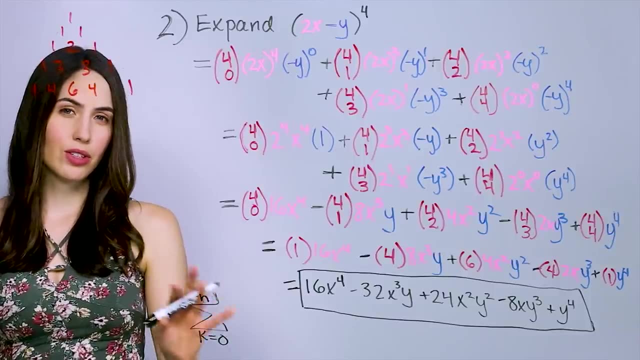 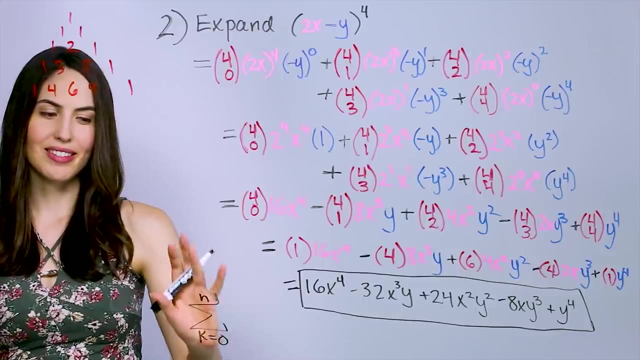 works for binomials- two terms inside. It doesn't work for trinomials- three terms, unfortunately. And by the way, if you see a version of the theorem that uses this notation, this strange one exotic Greek capital, sigma, sigma notation, it means the same thing as what? 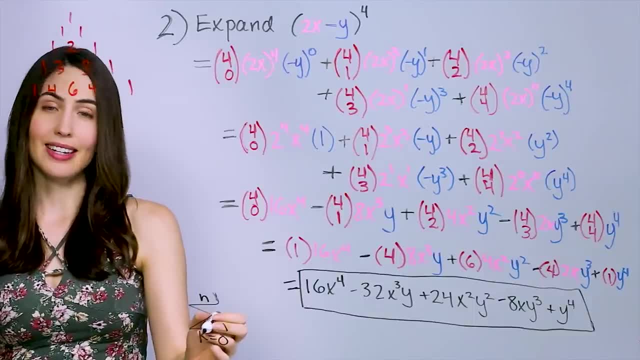 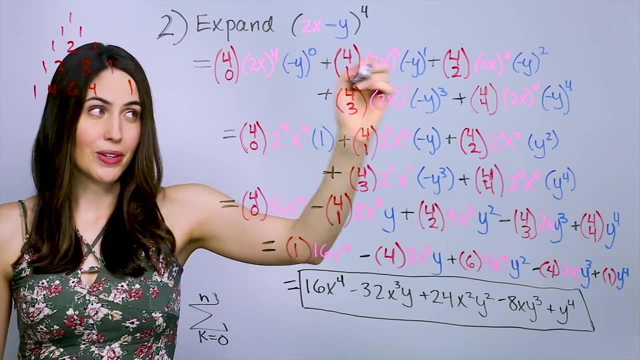 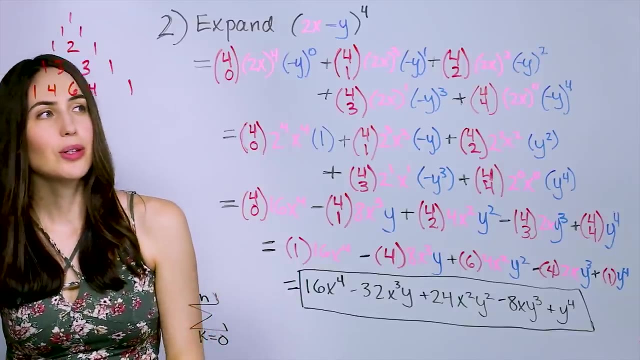 we were doing. I mean, this just means that K runs from 0 to N, that counter number which you already know, that it runs from 0 to N, that second term's power. So you can use that version if you want or if you have to, It just has even. 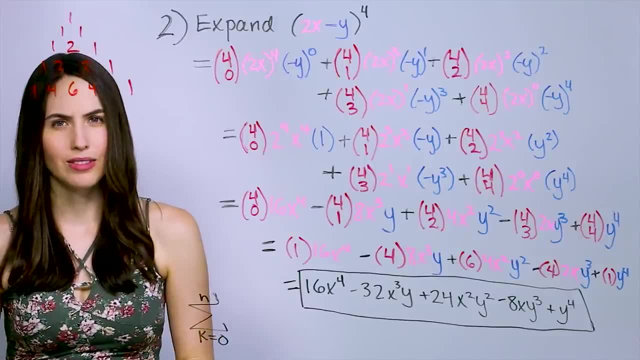 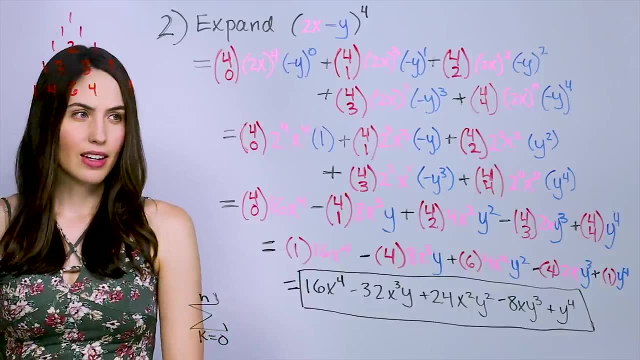 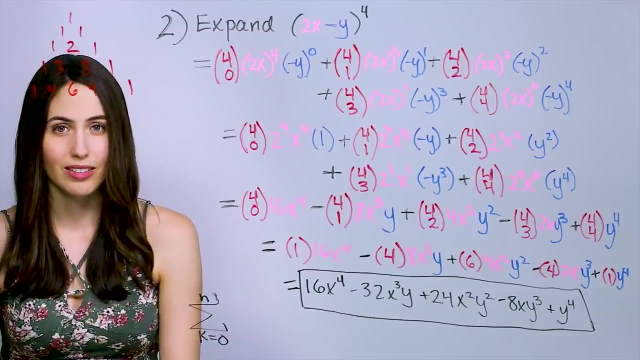 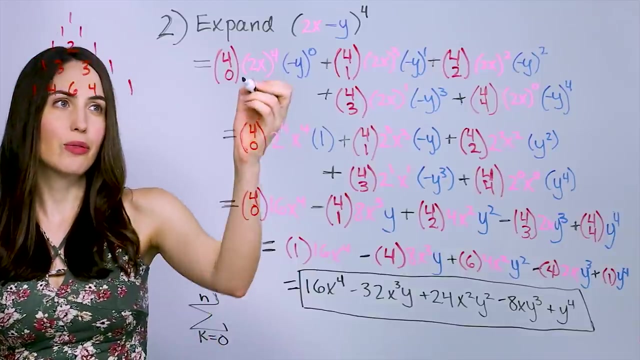 more formalness and notation, weighing it down unnecessarily. So if you understand what we did, you don't really need it. And then I would just say the biggest thing to remember with binomial expansions is just be careful. simplifying honestly Sounds dumb, but I mean, that's what trips people up with these like forgetting to. 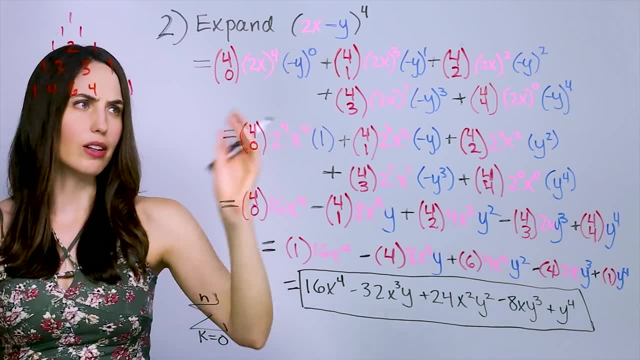 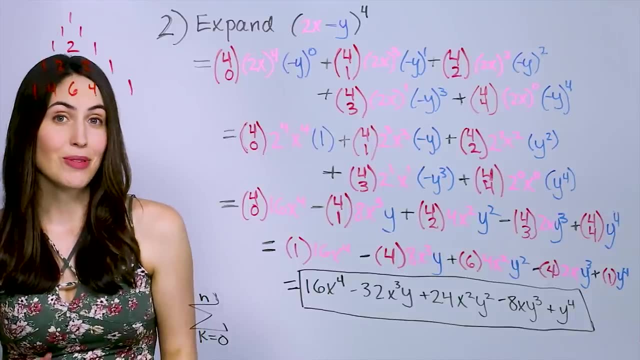 raise this number to the fourth power as well, or forgetting negative signs. keeping track of numbers, I mean it would be a shame if you understood the hard part of binomial theorem, how to set it up, and then you got tripped up by a. 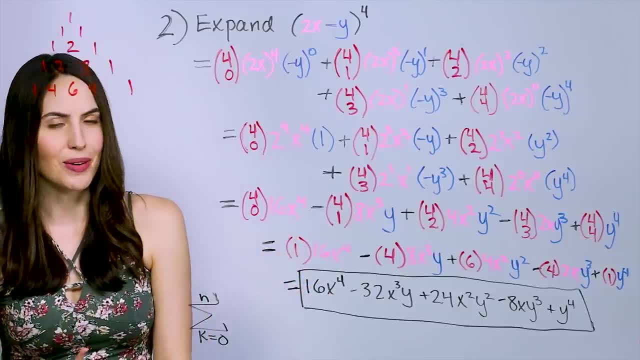 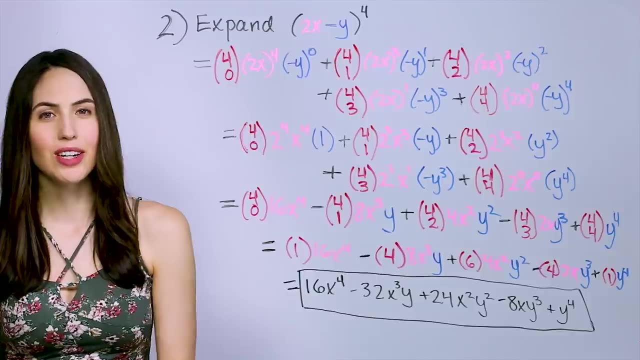 little simplifying details later. So I kind of can't remind you enough of that, because it just tends to be the thing that trips people up, So be careful. So I hope that helped you understand how to write out a binomial expansion with the. 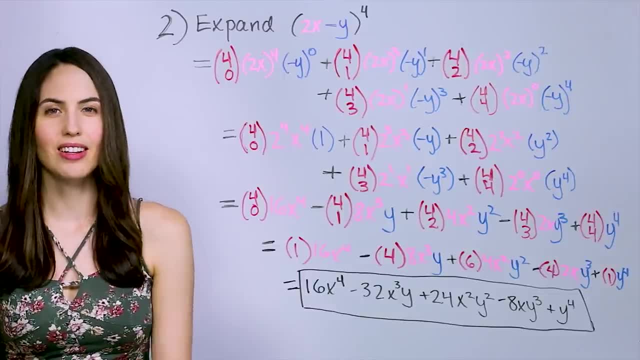 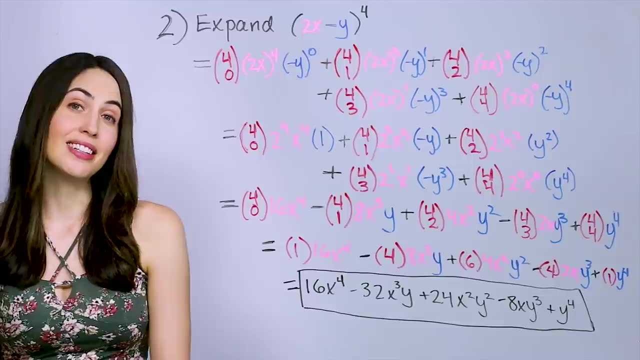 binomial theorem and or Pascal's triangle. I know this stuff can get kind of drawn out and tedious and a little rough that way You don't have to love it. But if you liked my video, please click like or subscribe.